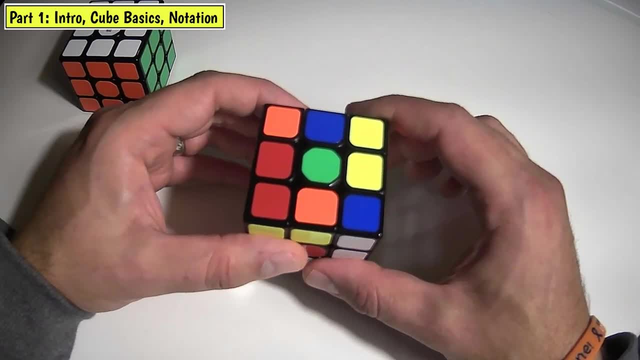 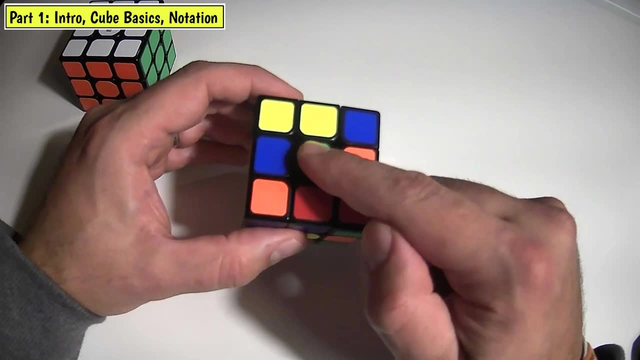 to this channel. I recommend that you watch this part. First off, we are going to start with the centerpieces, And because a cube has six faces, of course there are going to be six centerpieces, which you see there in the middle. The centerpieces- not everybody knows this, but those- 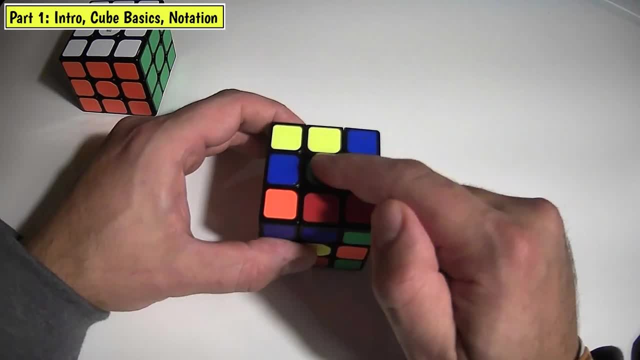 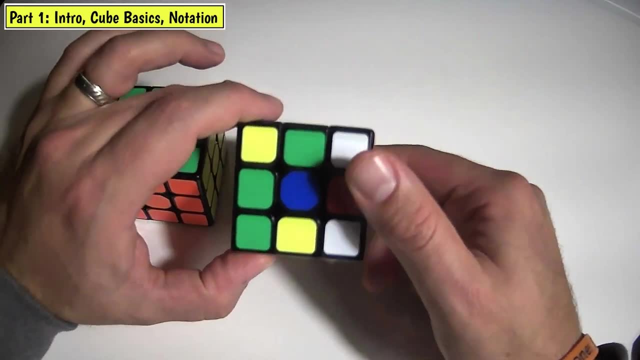 actually do not move Meaning once this cube is solved. this green centerpiece is where all the other green stickers will go. Opposite of green, you of course have blue. Same thing. If I flip this over to the other side, you can see that green and blue are opposite of one another. 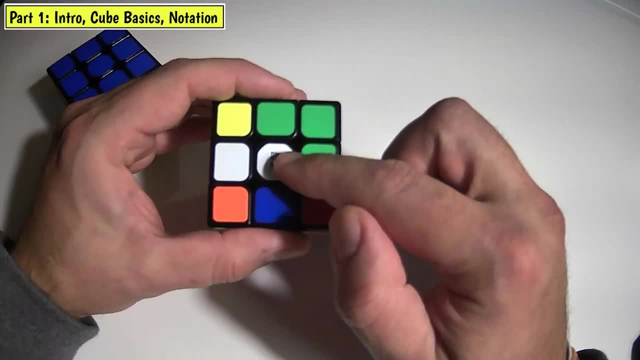 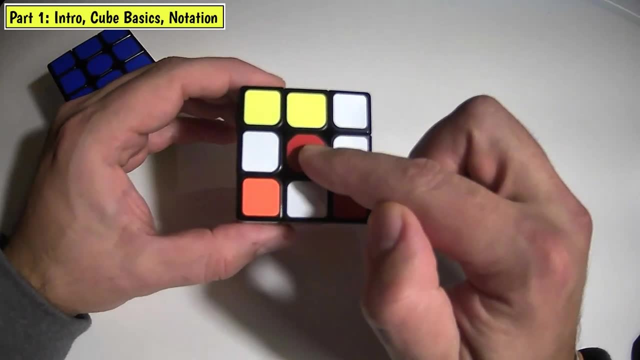 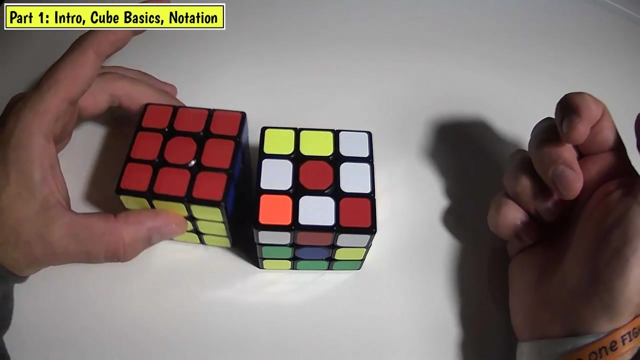 Next up we have our white center and opposite white is yellow and then opposite orange is red. So again, those centerpieces do not move, so eventually all of those surrounding tiles around that red centerpiece will also be red. Okay, the next part that we're going to talk about are the 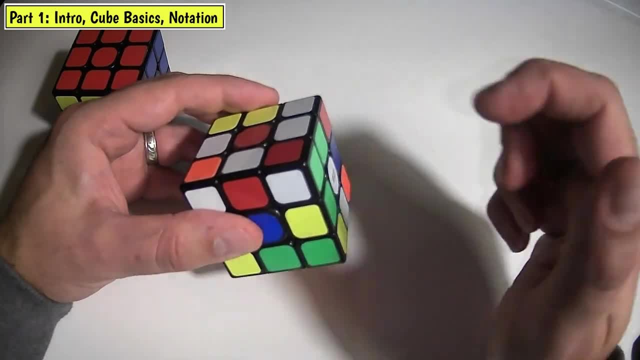 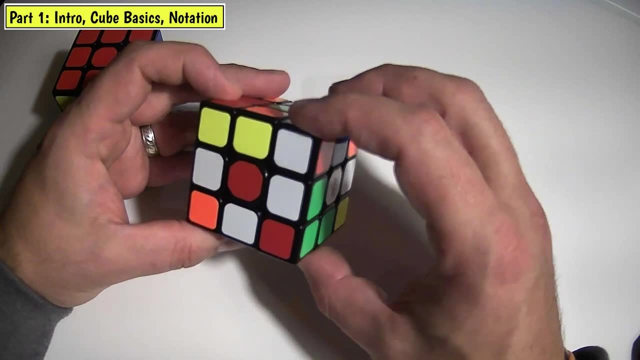 corner pieces And the corner pieces. just like there are eight vertices on a cube, there are eight corner pieces where you can see those three stickers. Okay, so there's a corner piece, and then there's a corner piece right there, right there, right there, and then same thing on the. 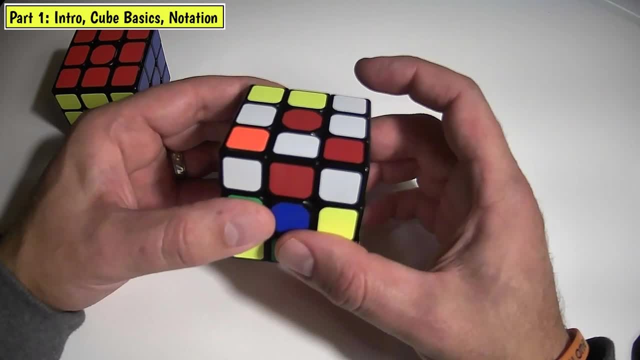 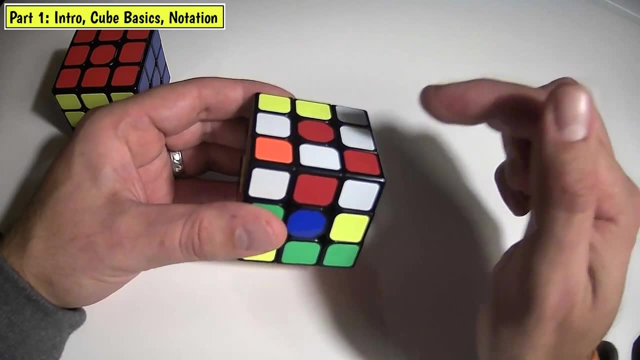 bottom. So there are a total of eight corner pieces. The last part that we're going to talk about are the edge pieces. So this example- this, of course, is an edge piece, because there are two different stickers on it. So the edge pieces are really in the center there. Anyways, again, 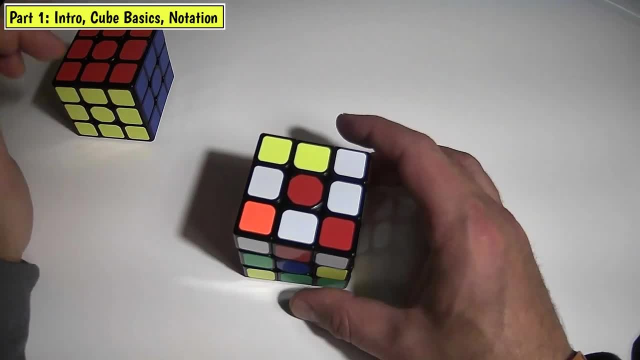 very, very basic stuff, but some important things that you're going to hear us talk about a bunch through the video. All right, so before we get into any of the cube notation, let's go ahead and let's talk about those six faces Here. I'm going to talk about the edge pieces and then 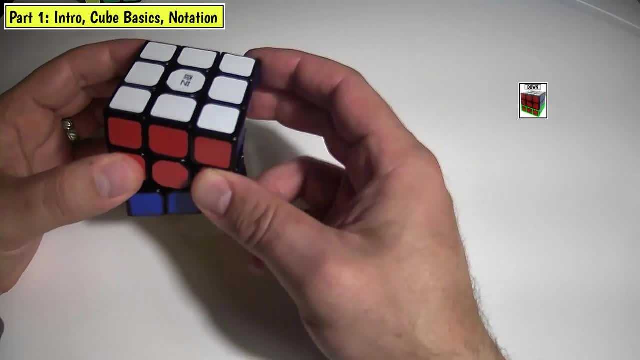 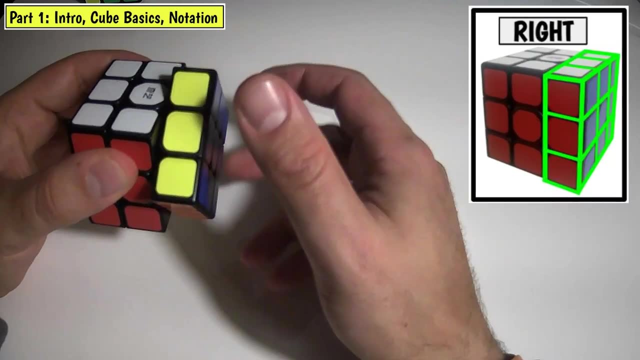 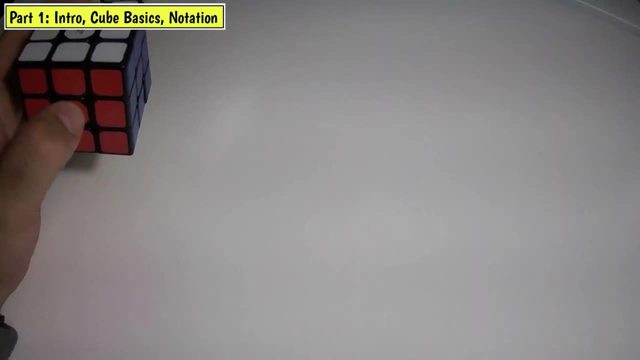 on top, of course, you see the up face. Then we have the down face, which I'm rotating right now. We have the left face, the right face, front and the back. Now, as we start to read, cube notation: 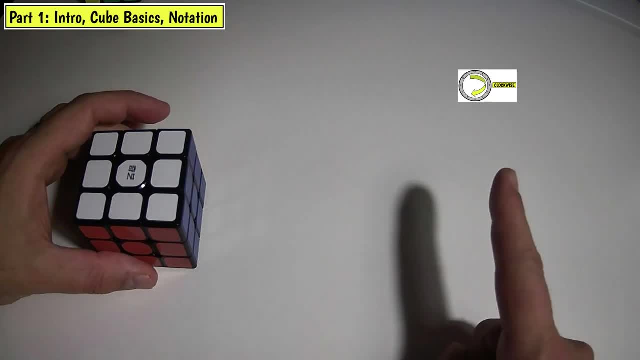 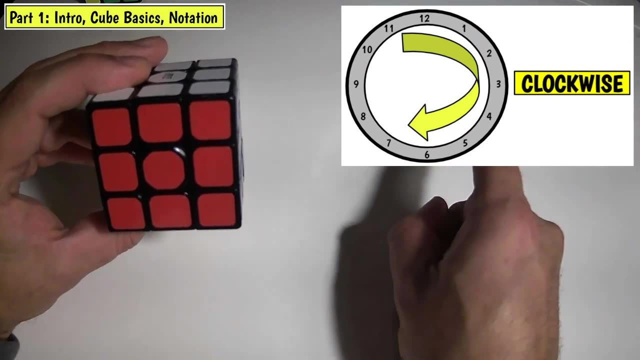 you will see sometimes, where you see the arrows in yellow, that means that you are going to be doing a clockwise movement And clockwise means- if you imagine over here I've got a picture of a clock- Clockwise means that you are turning it the same way a clock would turn the hands on a. 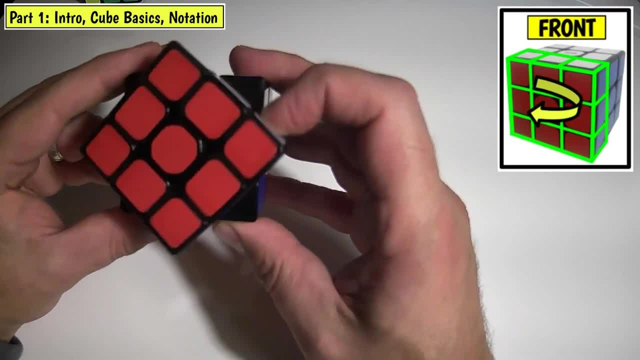 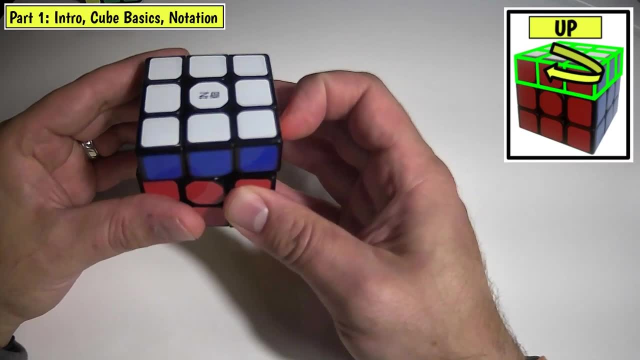 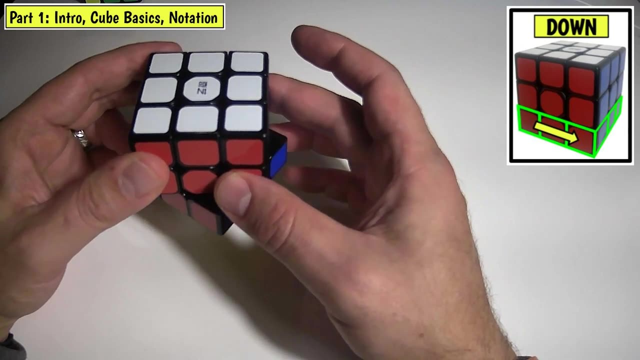 clock. So when we see F, just the letter F, it means that we are moving the front face one time. So if we were doing up, we just rotate it like this. Okay, so then down, like you can see. we see the arrow that is moving it down. We see left- it's just like this- and right. 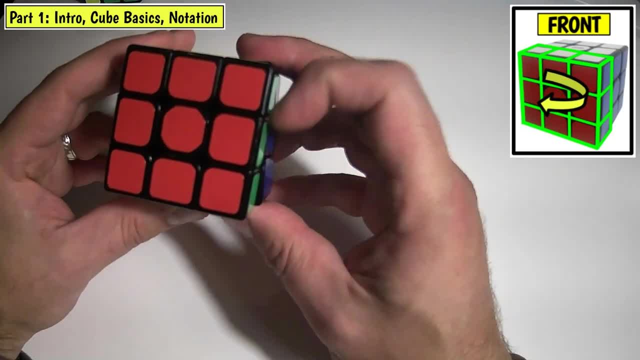 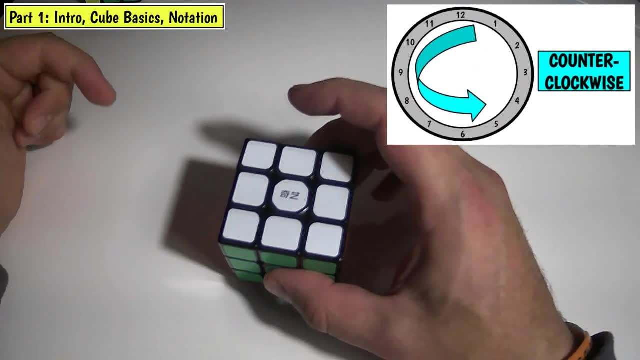 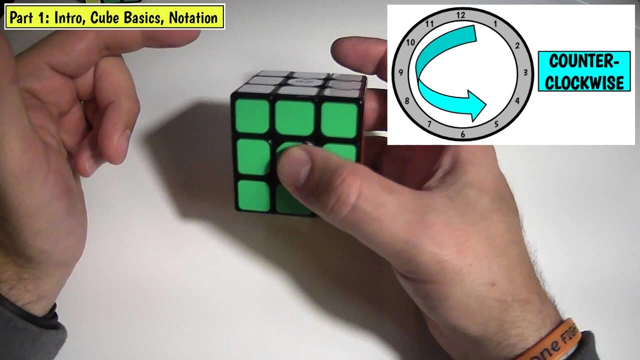 And then front and back. Okay, so now let's get into talking about some of the counterclockwise movements. Sometimes they're known as prime, sometimes it's called inverted. Throughout this video, I'm going to say inverted, which means the opposite direction. So now, instead of moving the 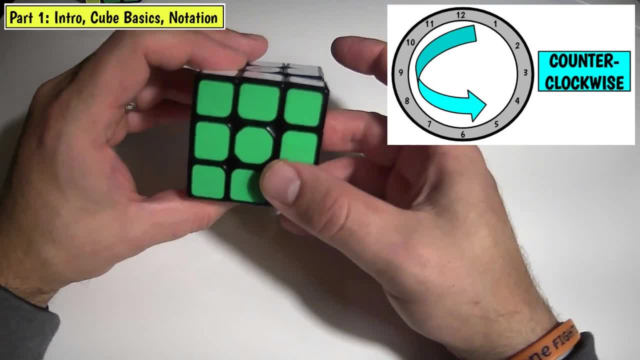 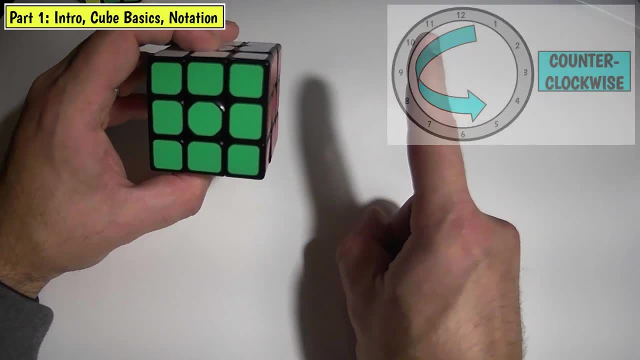 faces in a clockwise direction, like we just practiced, we are going to be moving it in a counterclockwise direction, which means the opposite direction. So now, instead of moving the opposite of how a clock spins, So let's practice, just like you can see off to the side here. 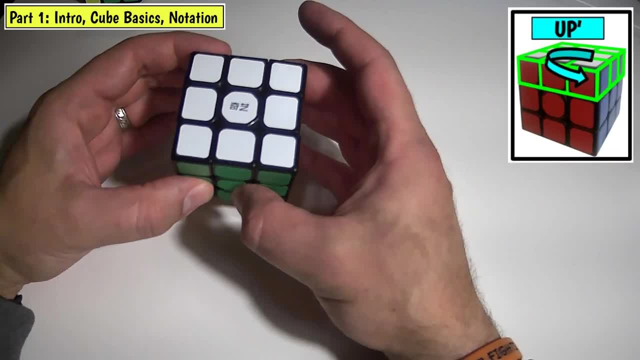 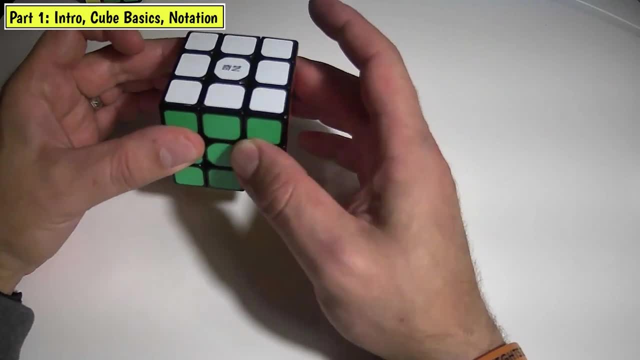 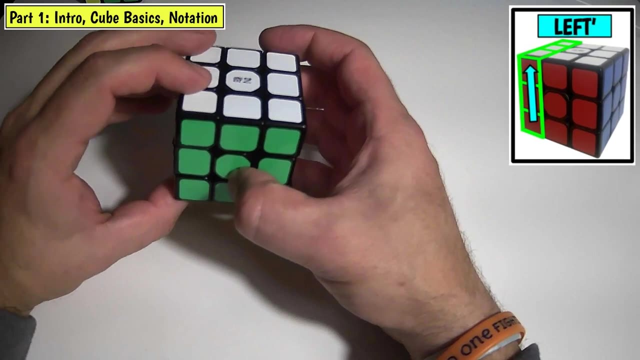 let's practice some of these inverted moves. So up inverted starts by just going this way. So we're going opposite, counterclockwise, Okay. so down inverted. just like you can see with the arrow, we're going to be shifting the bottom face. Left inverted looks like this: There's one, two, four. 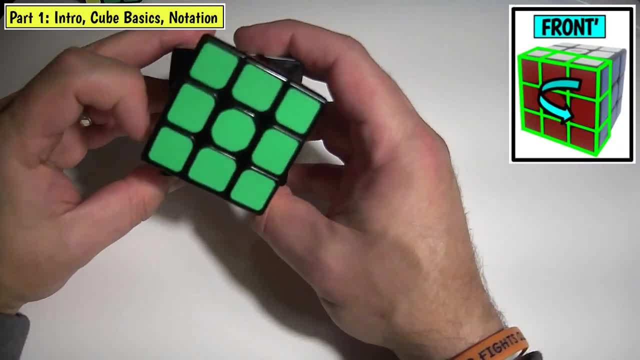 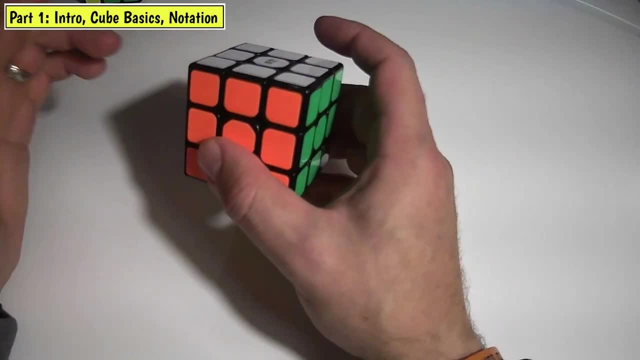 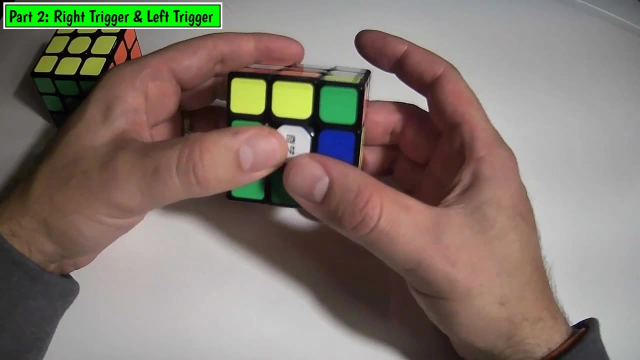 Right inverted and then front inverted and finally back inverted. So again, as we go through each of these different steps with the algorithm, you will see that as I'm modeling it to the left, I will have all of the different directions posted there on the right. All right, so now we're going. 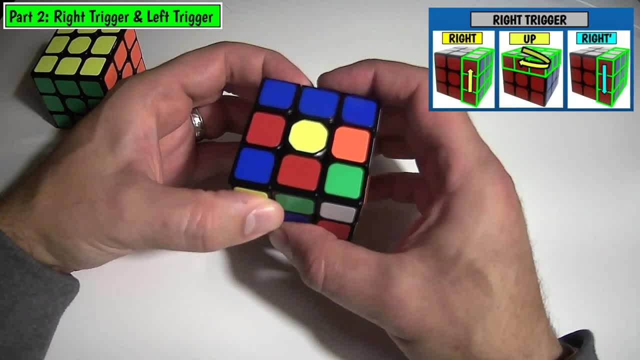 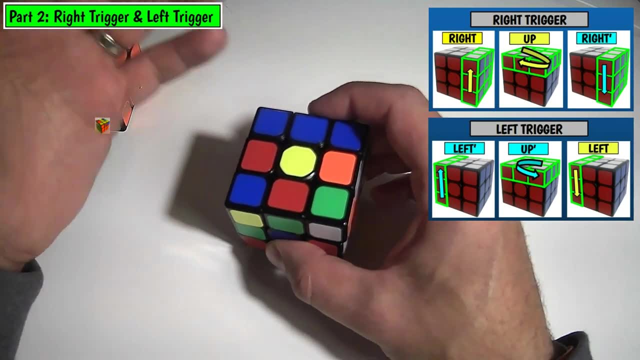 to actually learn part of our first algorithm, which is called the right trigger and the left trigger And, to be completely honest, if you can master the left and right trigger, you can actually knock out like the first four or five steps of the algorithm. So let's go ahead and 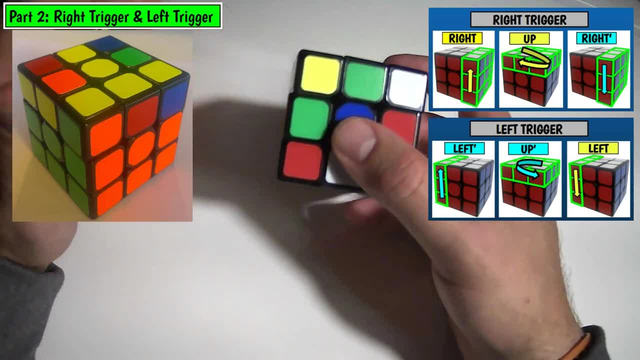 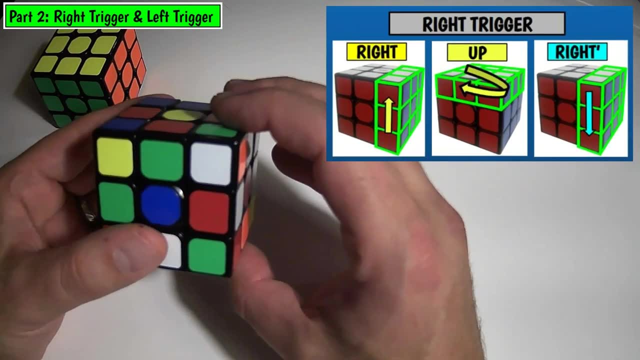 see if we can get to the middle layer, And if you can do that, you can really get all the way up to the middle layer, solved just by knowing the right and left trigger. All right, so to perform the right trigger, you're going to follow these steps, like you can see over here where we are going to. 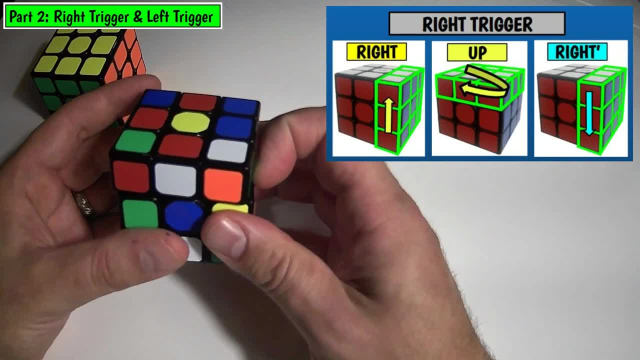 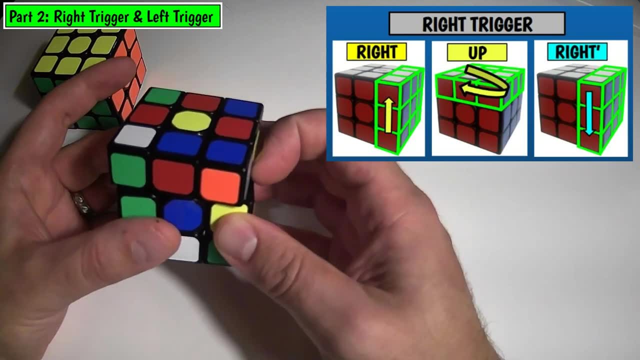 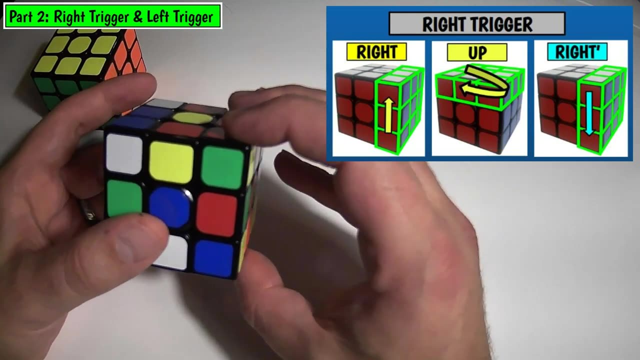 go right up, right inverted, And I'm going to do that again. So we have right up, right inverted. I'll do it one more time: Right up, right inverted. And the more and more you're going to do this, the more you're going to get to the middle layer, the more you're going to 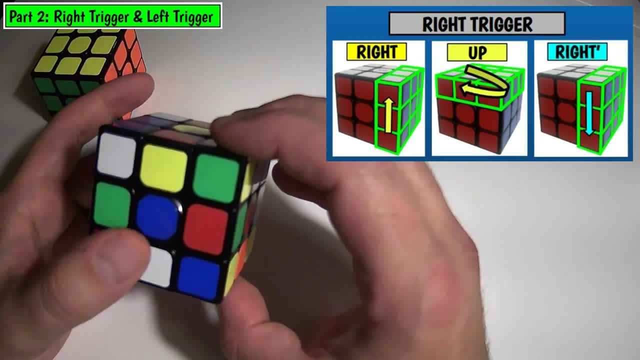 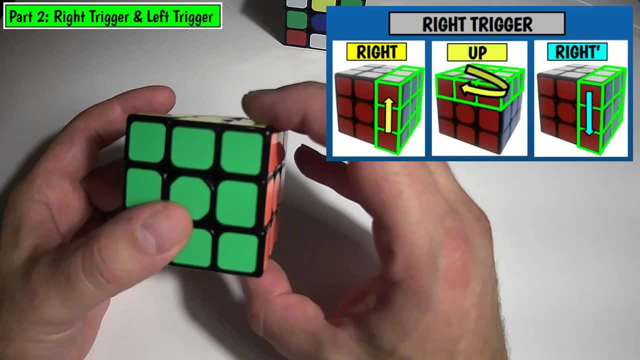 practice it, the right and left trigger become just super, super natural and you can execute them really quickly. For example, let me just show you here: on the solved cube, I am going to do the right trigger four times And when I've done it four, on the very fourth time, you will see that 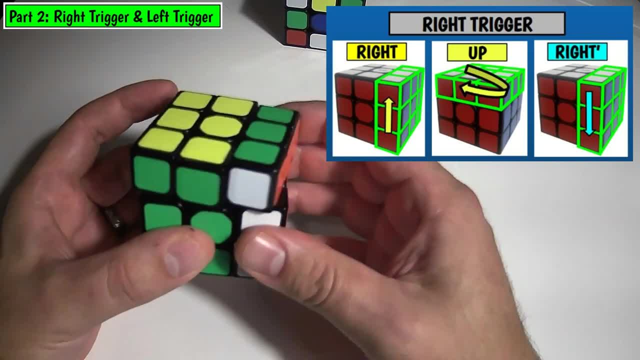 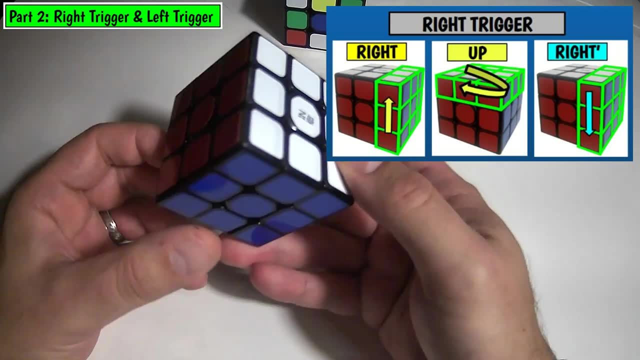 my cube will be back to solved. So example: So there's one, two, three, four and it's back to normal. And the other thing that's kind of cool. let me grab a dry erase marker. I want to show. 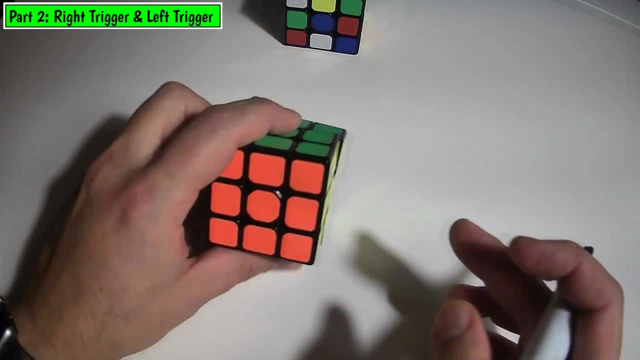 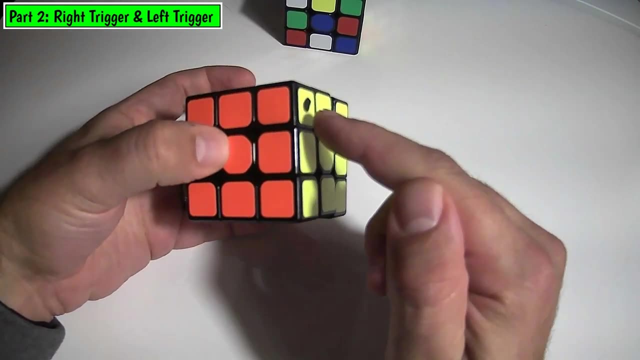 you something? Okay, so what I'm doing is I just drew a little dot on that corner After I do the right trigger once this black dot is going to be right here, And this is an important skill that y'all are going to see once we get into trying to solve that middle layer. So, if I do it again, 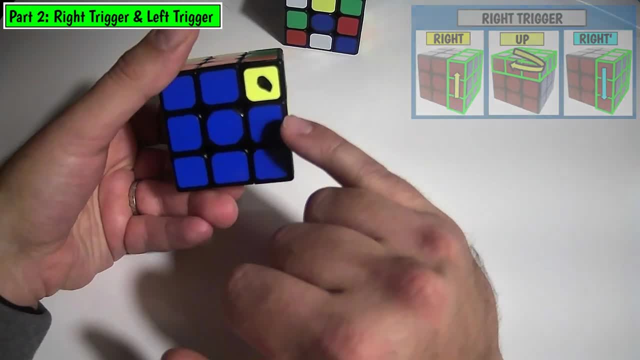 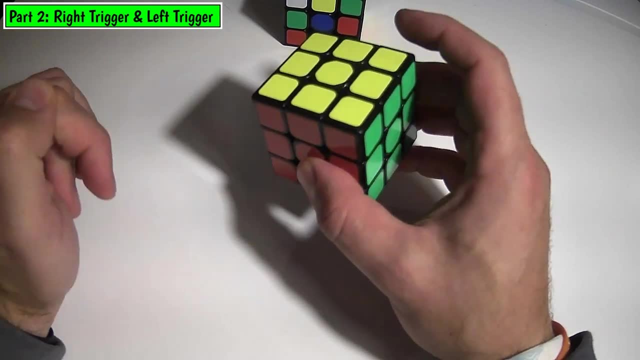 right up, right inverted, Just like I told you. there it is All right. so now let's check out the left trigger. Now I am right handed, So the left trigger I cannot execute as fast as I can the right trigger, But again, I practice it. So I'm going to do that one more time And when I 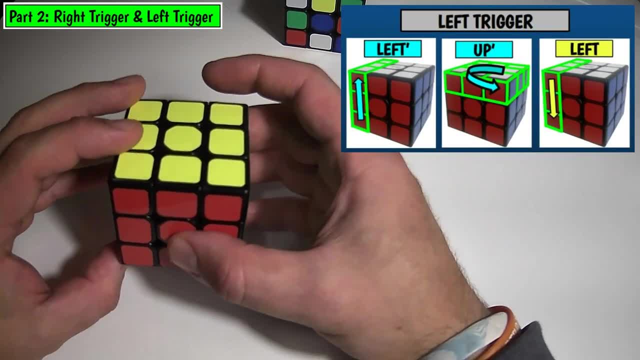 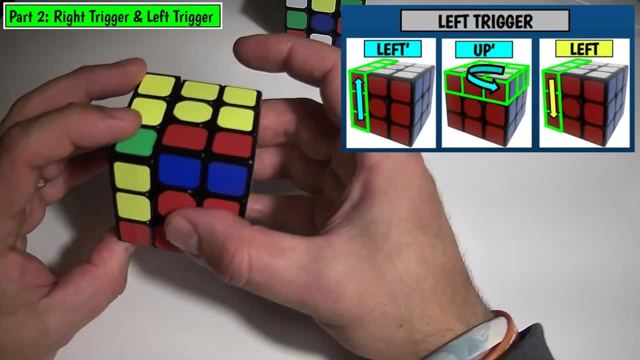 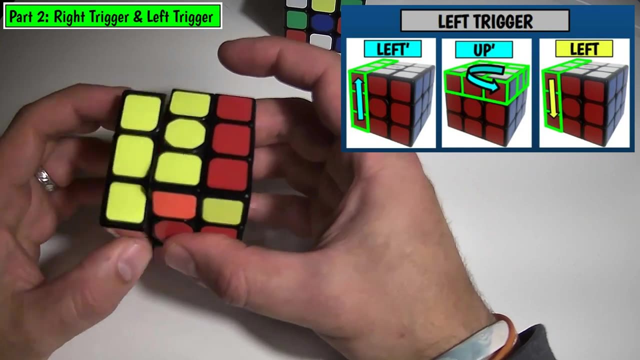 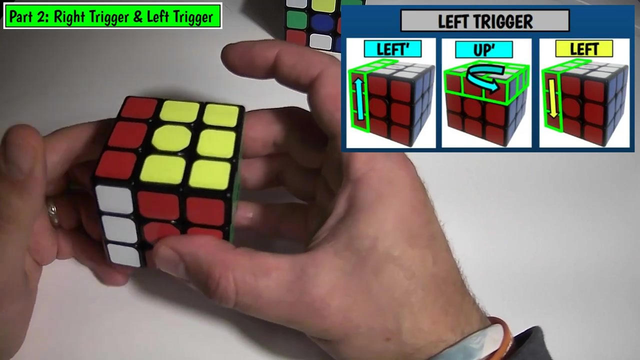 practice it so many times, it comes pretty quickly. So to operate the left trigger, you are going to do these three moves. We have left- inverted up- inverted left. I'll do it again: Left- inverted up- inverted left. Left inverted up- inverted left. Left inverted up- inverted. 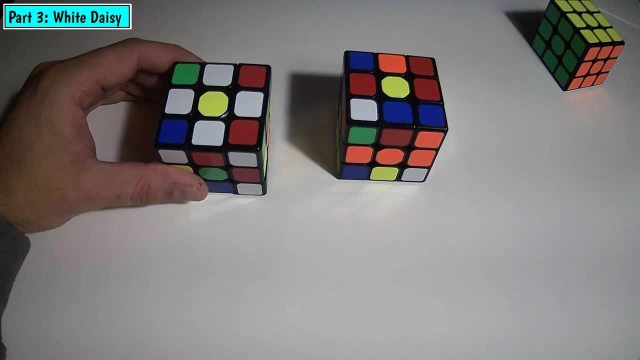 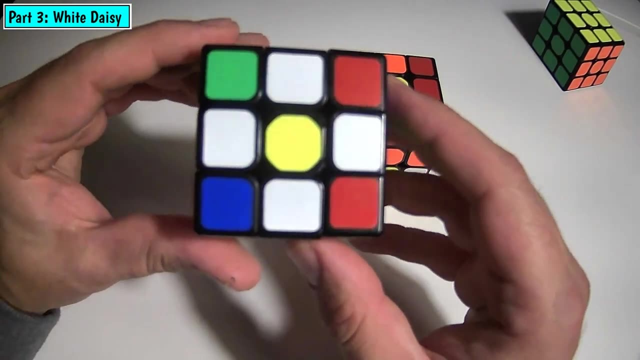 left. Okay, so now we've practiced some cube basics and learned some of the cube notation and the right and left trigger, Let's go ahead and start step one, where we are trying to make the white daisy. So to complete the white daisy, you're going to have your yellow 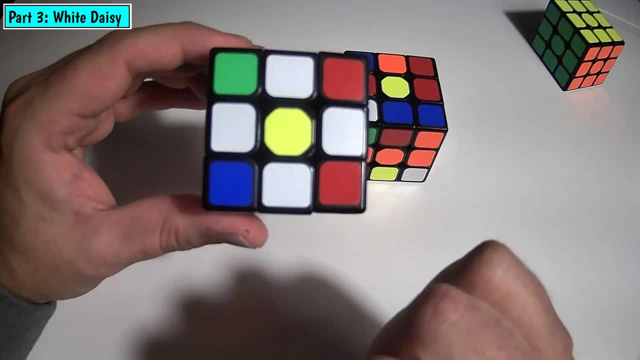 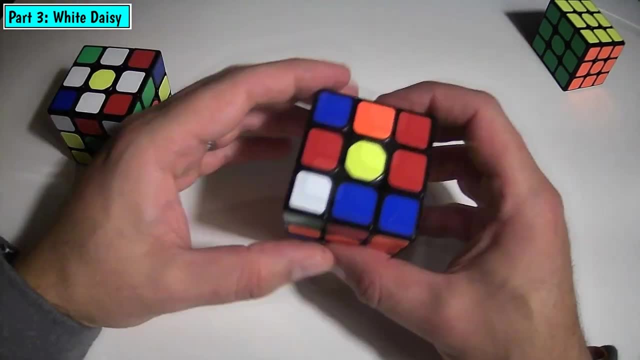 center piece surrounded by four white edge pieces, And, as we go through and practice this, if you have white corner pieces in there as well, do not worry. So this is what we're trying to make Now. this was a step that, honestly, was very difficult for me when I first started learning to cube. 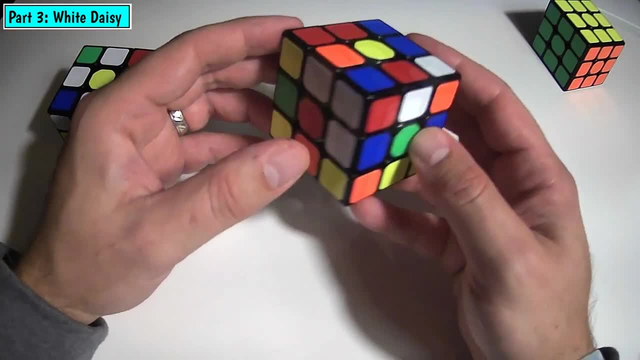 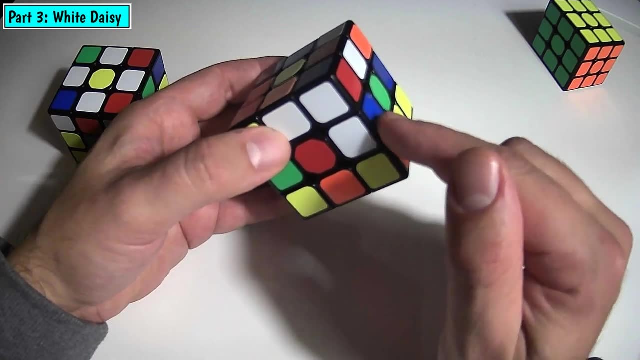 And now it probably takes about five seconds or so to complete. So what I'm going to do is I'm going to kind of rotate my cube Around until I see white edge pieces. Remember, like we said earlier, white edge pieces have two. 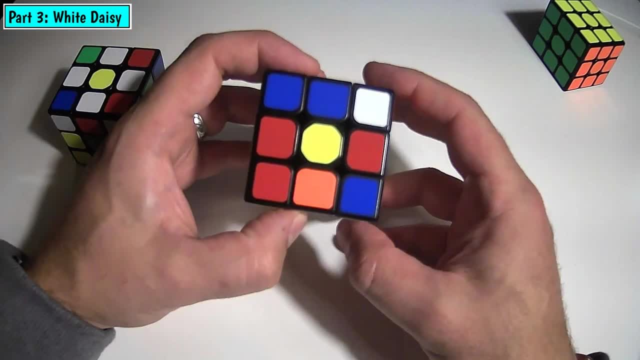 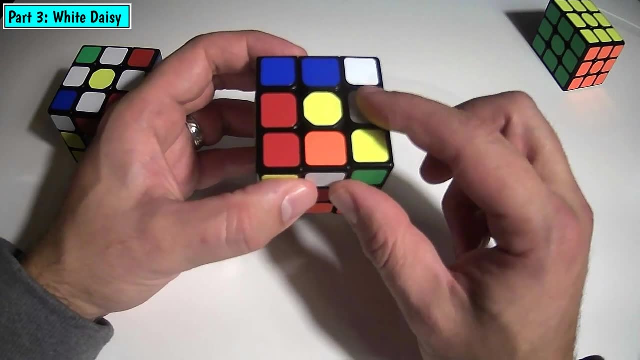 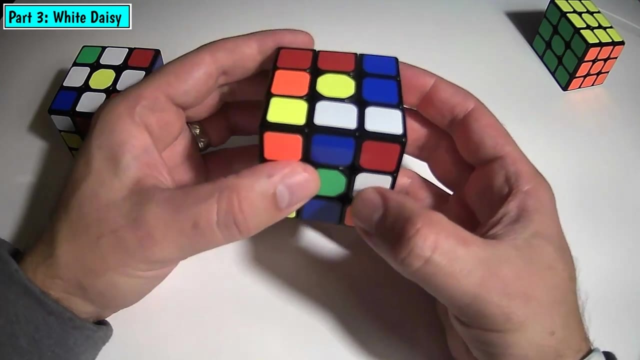 stickers on them. For example, I can see that this is a white edge piece. Now, to get this white edge piece in place, all I need to do is turn the right face like that. All right, so there, we've got one of the four petals in place. Let me kind of look around see if we see any other ones. Sure enough. 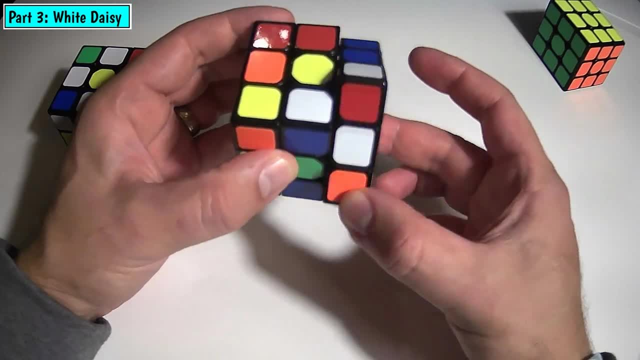 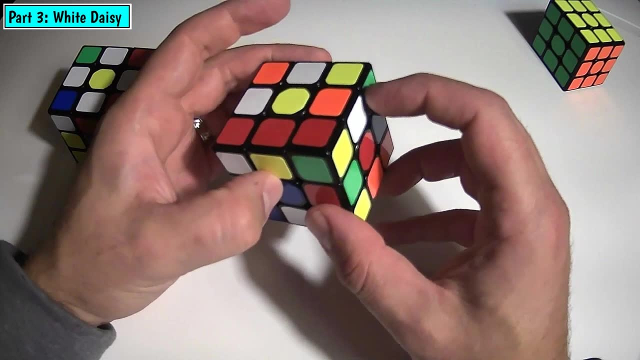 there's a white edge piece And again, this is a pretty simple one. All I need to do is turn that right face. So I keep scanning, try and find one. Okay, so here's a white edge piece, But you can see. 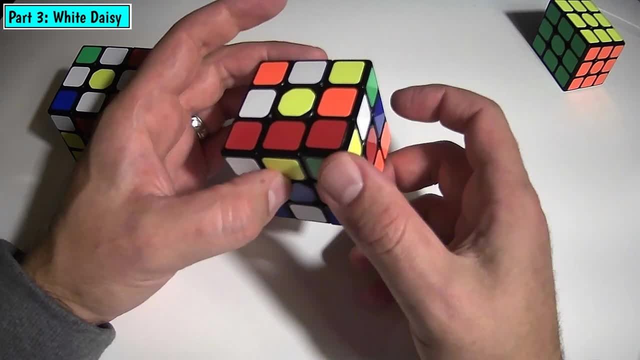 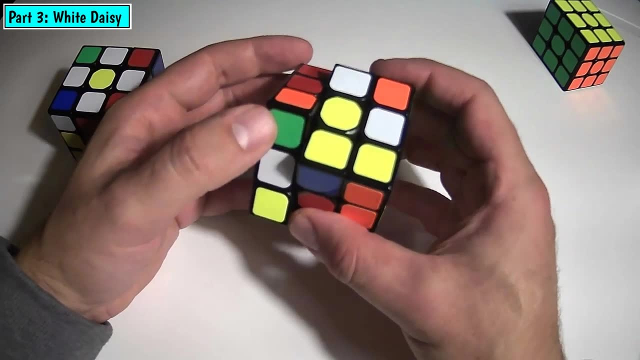 that it is. it's not going to just line up perfectly with one rotation. So what I'm going to do is I'm going to actually turn this face once, like this, And then all I need to do is bring it up And oh. 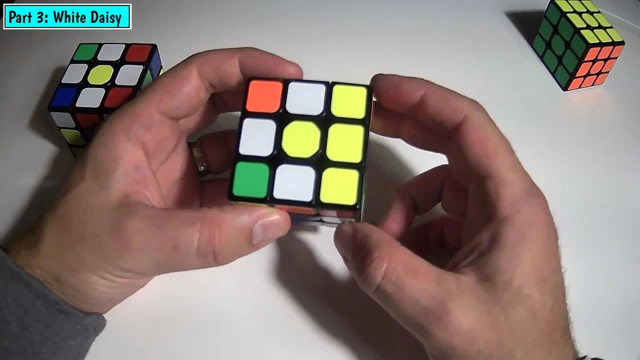 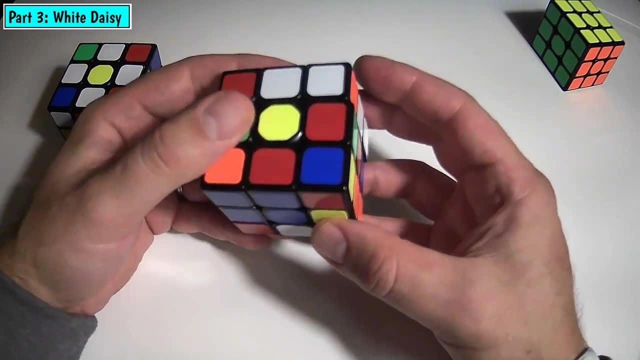 my goodness, now this worked out pretty well. All I need to do here turn that right face And there I've made the white daisy. Like I've told the third, fourth and fifth graders in my club, they were so proud of themselves for making the daisy, I gave them a high five. I said. 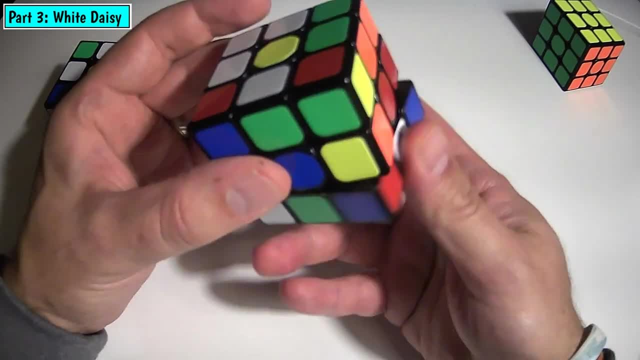 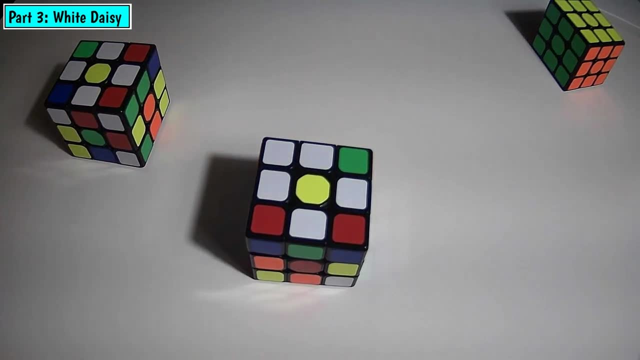 that's awesome. And then I grabbed their cube, scrambled it up and told them to do it faster And, honestly, that's the best advice I can give you as well, if you're watching this at home. If you just keep moving on with this video, I don't I doubt you're going to retain a lot of. 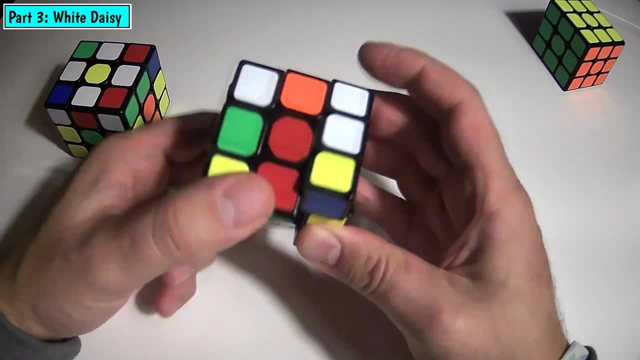 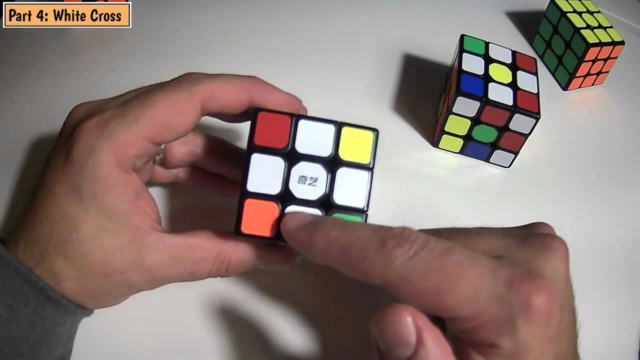 what you're watching. So I would really, like I said, just keep on scrambling that cube up and just continue to make the white daisy over and over and over. Okay, so for the next part of this video, we are going to be trying to make the white cross, as you can see. 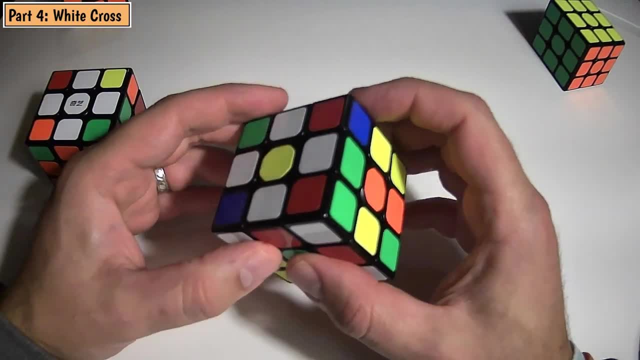 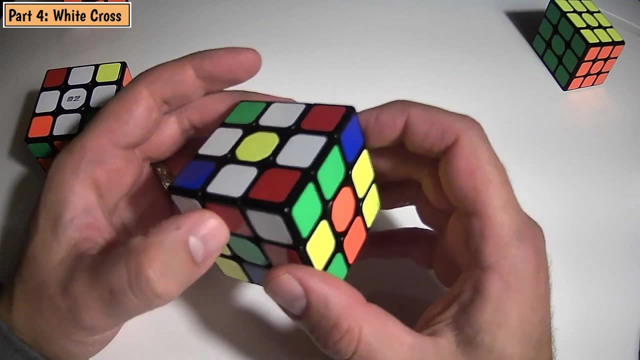 So let me grab my cube. I just made the white daisy on, So what we're going to be doing is we're essentially going to be bringing these white edge pieces down so that they're on the bottom, But there is one little trick here, Okay, so let me just start right here. So we got to get this white. 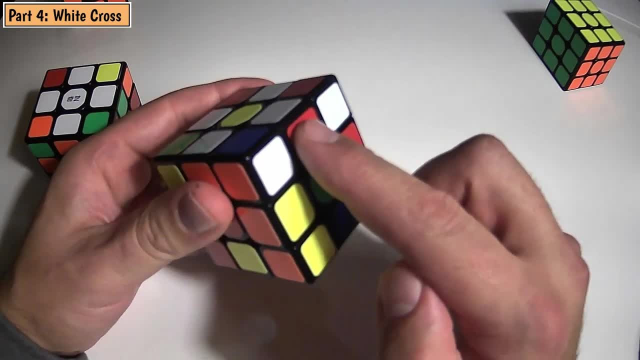 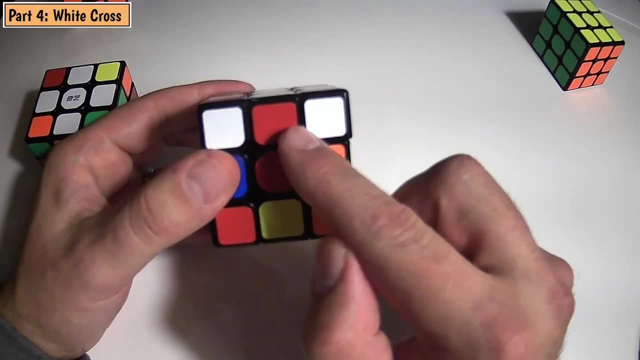 edge piece in the right spot. Now, if I look, I can see that we've got white, red and then green. That does not match. I need to rotate the top face until we see these edge pieces meet the red center. So now I see white, red, red. 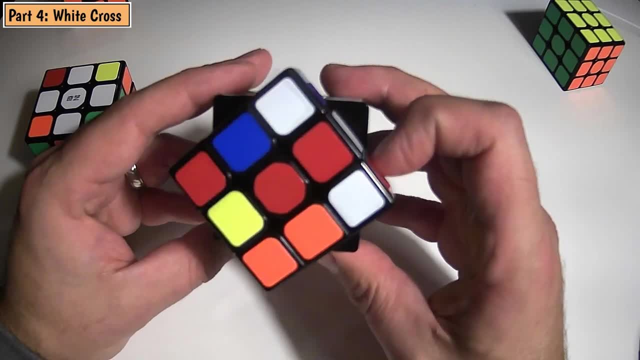 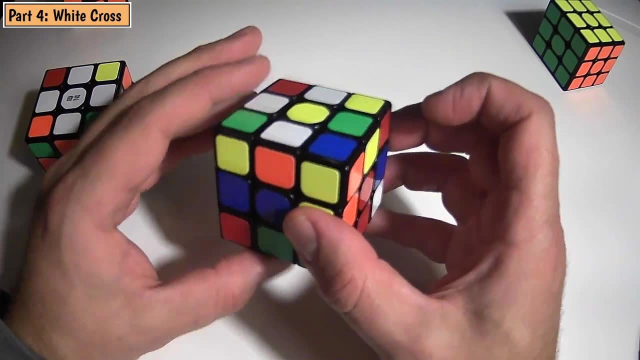 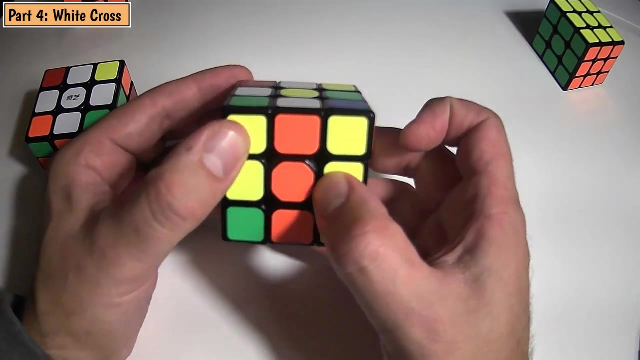 And that is in the correct spot. So what I'm going to do is I'm going to rotate the front face twice until that white edge piece is in the right spot. If I move it back to my top, you can see that now I see white, orange, blue. I'm going to rotate this top face until that matches up perfectly. 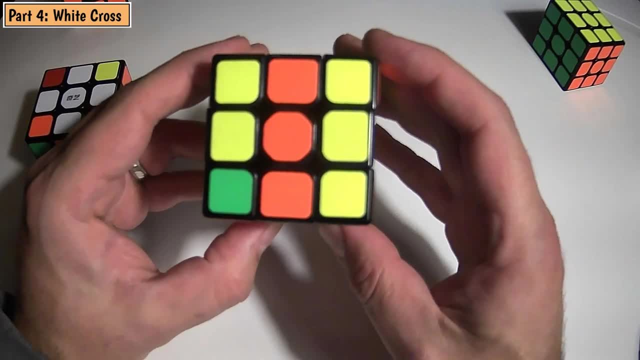 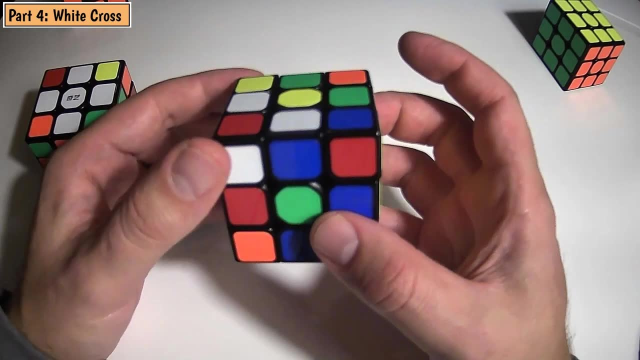 where we see white, orange, orange, And again, I'm just going to rotate that front face twice. There's one, there's two and now that's in place. If I move it back to my top, this does not match. We see a white, blue, green, So I'm going to rotate. 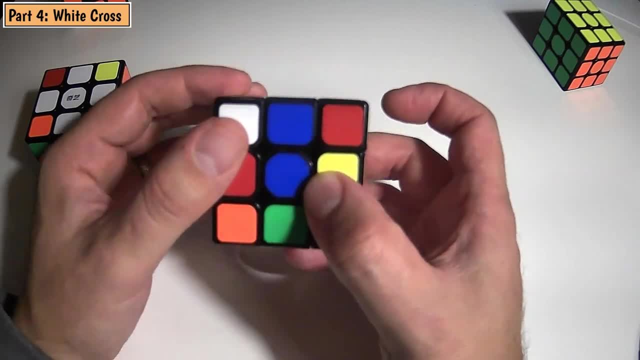 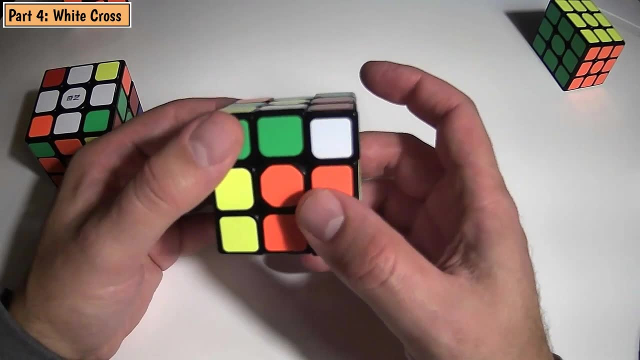 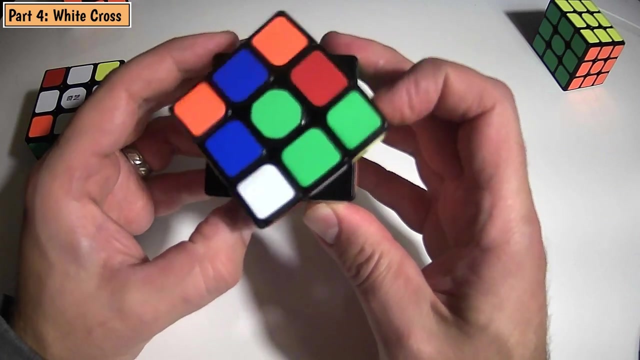 this until that matches, There we go. We see white, blue, blue. Rotate this twice. Now we've got three of the four parts of the cross And the last one I need to do is I just need to rotate this like that That matches White, green, green And there you can see that we've made the white cross. 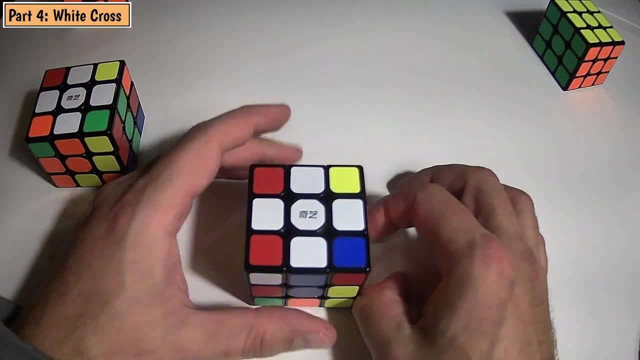 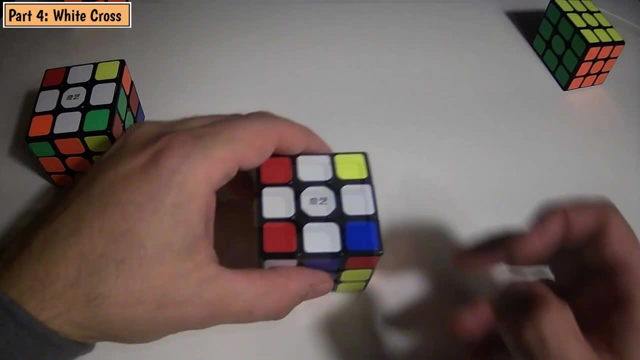 Now, as you're going through and solving this, if you have any of the white corner pieces matched up as well, don't worry. It doesn't actually have to make a cross if you've got some extra parts in there again. Just same thing I said with the white daisy. Again, I would 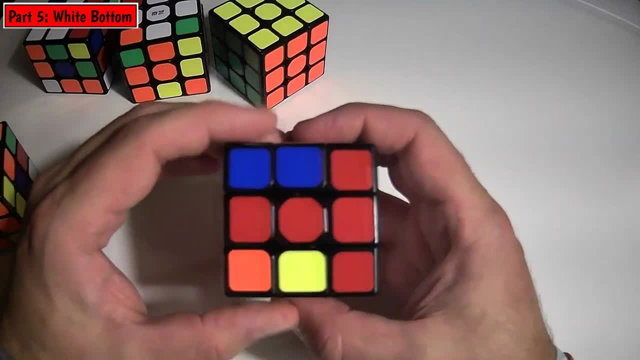 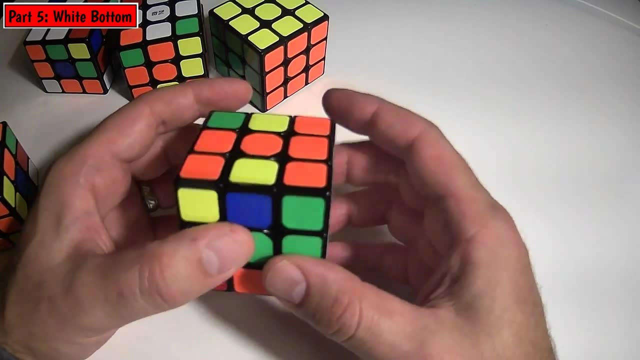 recommend scrambling this thing up and doing it again. All right, so this next step. what we're going to do is we are going to actually complete the white bottom, And along with getting the white bottom complete, you can see that the bottom layer is also completely done. Now this, like I told you, 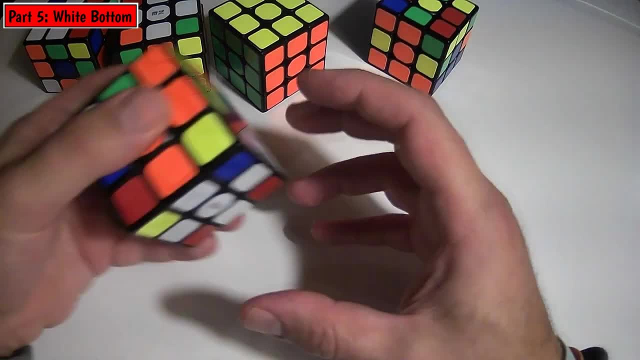 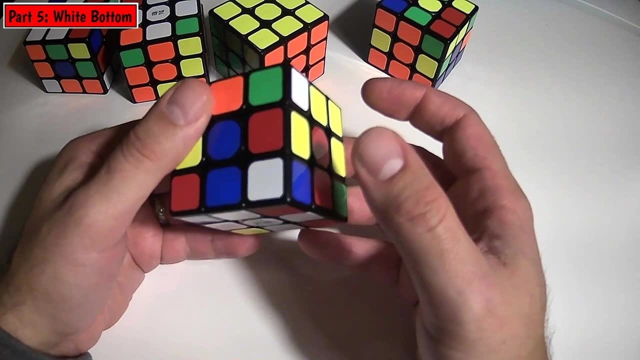 earlier. this is where knowing that right and left trigger is going to come in really, really handy. We've got the white cross. We want to make this entire bottom white, Okay, so what I'm going to do is we need to find the other white corner pieces. So there's one right there. there's another one right there. 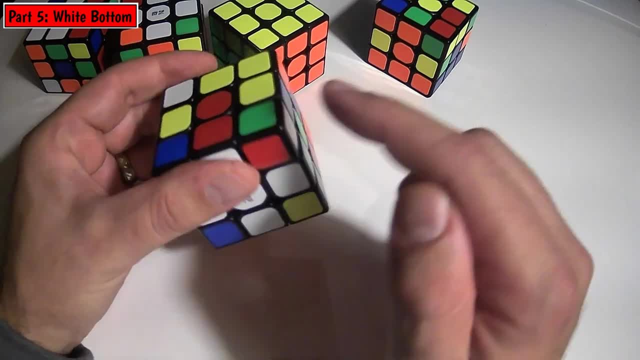 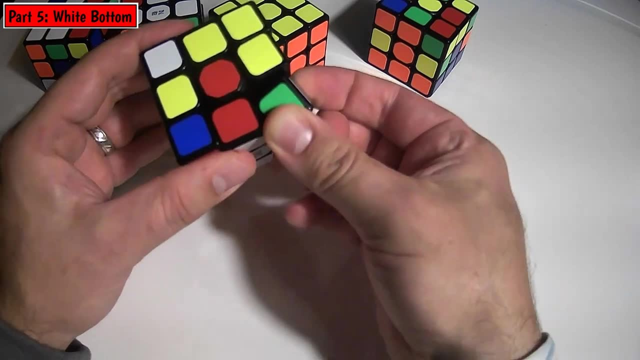 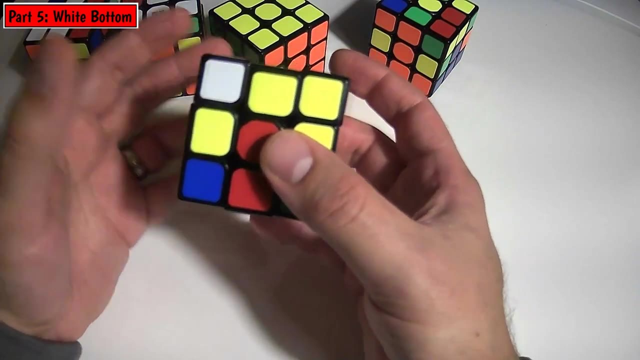 there's one that I'm missing, and then this one. Now I shouldn't have to mention this, but do not ever, whether using one of my cubes or one that you have at home, do not ever try to rotate these corner pieces to try and get them the way you want them. Sometimes kids try and take. 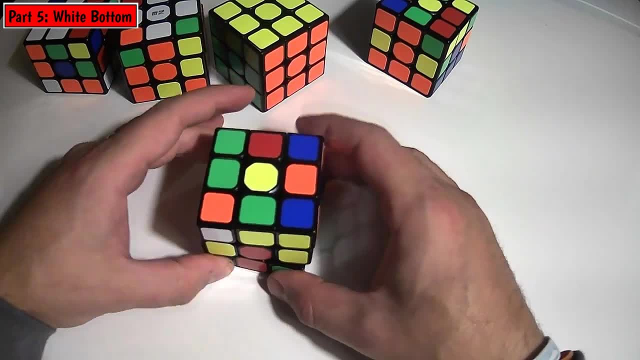 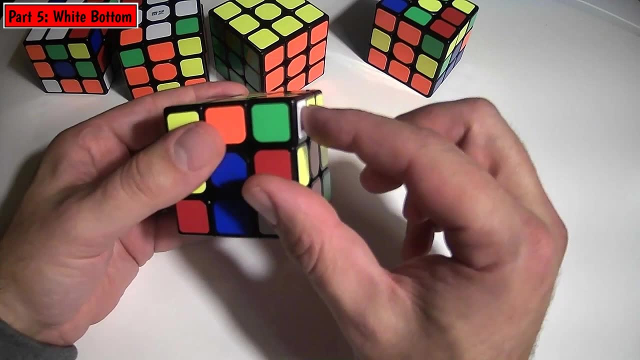 apart the cube and twist the pieces like that. that is not how we're going to solve the cube. so what i'm going to do, i'm going to start with this white, green, orange corner piece. what i want to do is i want to match up this green with the center piece that is also green, so we see a diagonal. 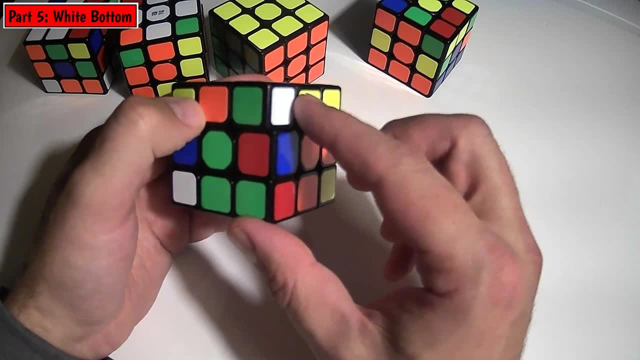 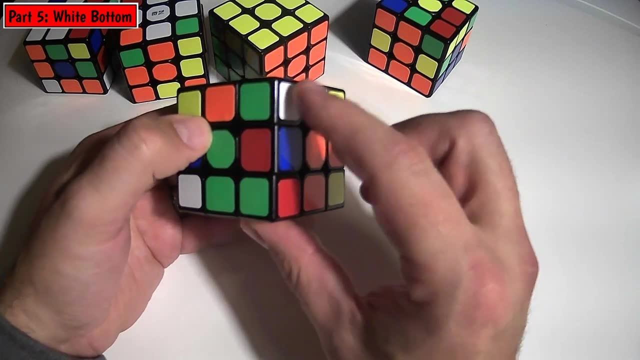 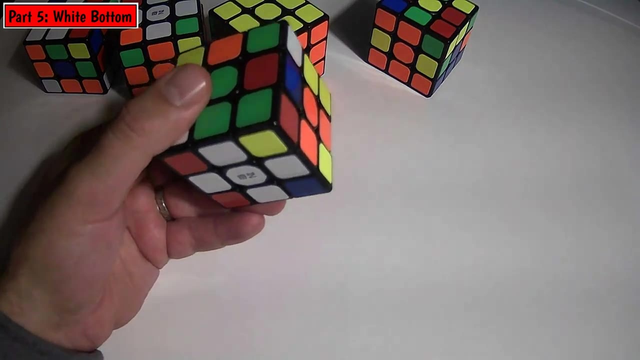 connection. so, for example, there we see the white green, green diagonally. now, if you remember earlier, when we did the right and left trigger, this white corner piece, after i perform the right trigger, once this piece is going to magically be right there. right, so, to do the right trigger, i'm going. 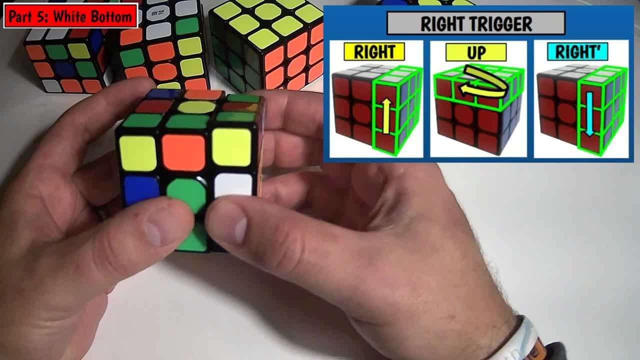 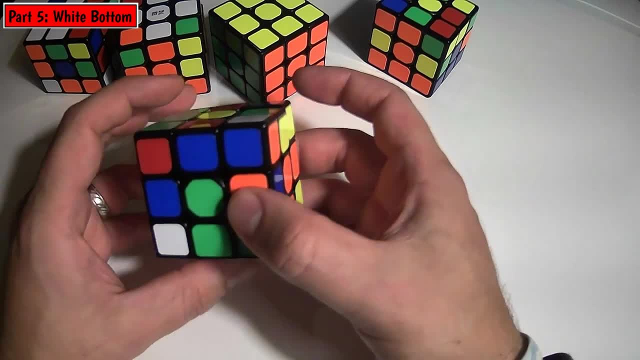 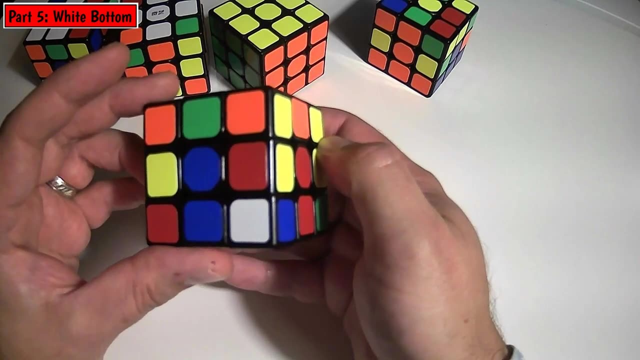 to do these three steps again. so i'm going to go right up, right inverted, okay. so now i'm going to look to see if i have some other white corner pieces with, you know, the white sticker being here, and in this case i don't have any that are up in that. 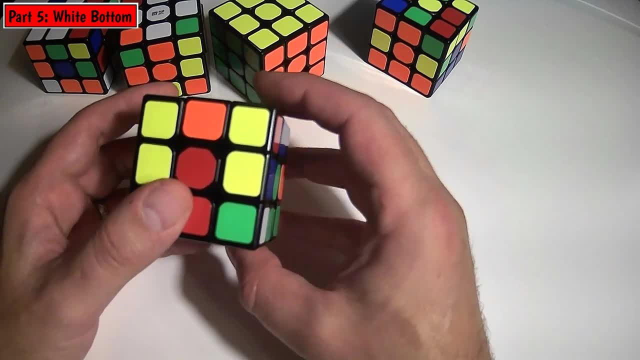 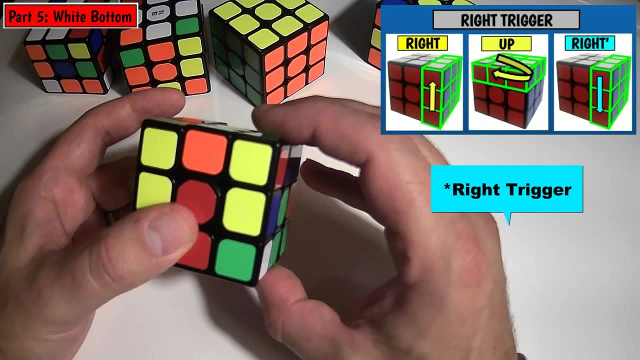 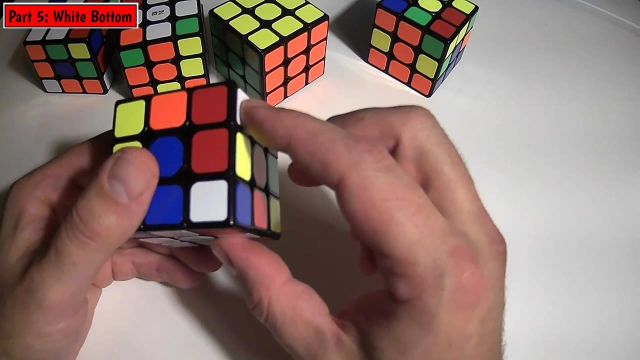 position where i want it. but again, like i said earlier, that right trigger, left trigger is going to come in really handy, okay. so to get this piece up here on top, do that white trigger again, so i go right up, right inverted, okay. so now i've got that white corner piece up where i want it. 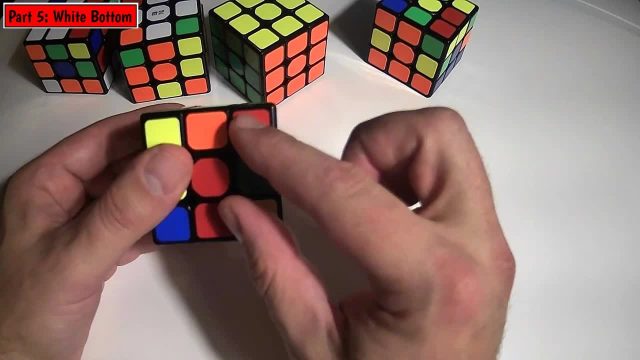 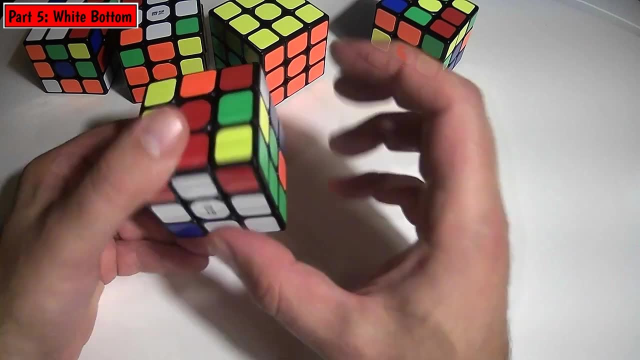 so i'm going to rotate it again, just like we did before. so now we have white, red, red diagonally, and i'm going to do that right trigger again. so after i do the right trigger once, it'll magically be there. so i'm going to go right up, right, inverted. 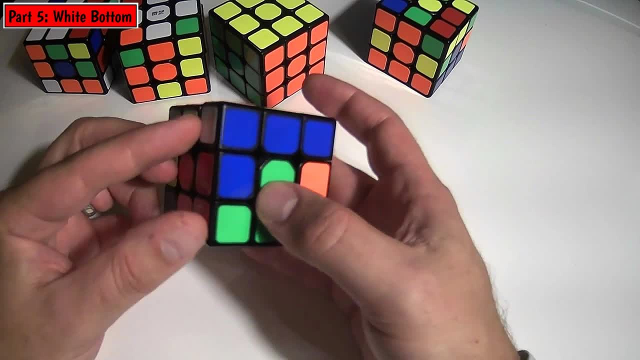 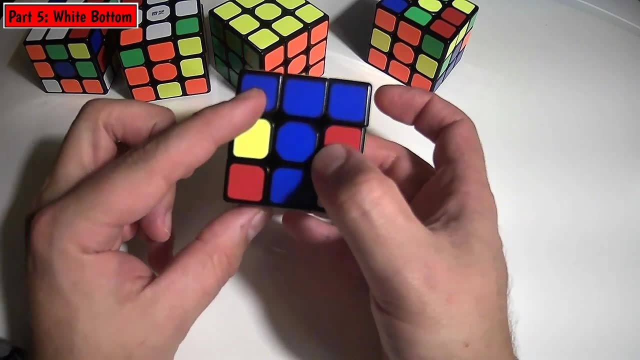 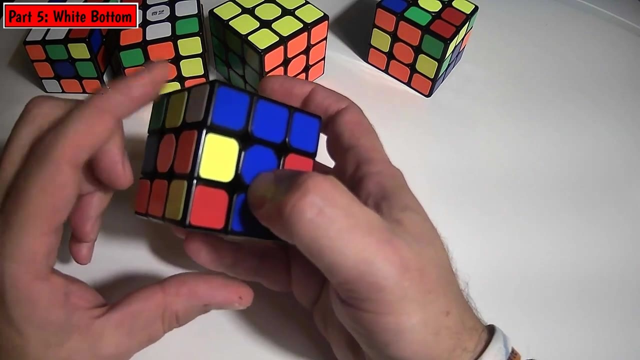 all right, so i always have two more to go. okay. so here i keep scanning and there i see a white blue. but remember, we want that diagonal connection. so white blue, blue this time around. because the sticker is on the left, i'm going to do the left trigger. so this piece when i'm done with the left. 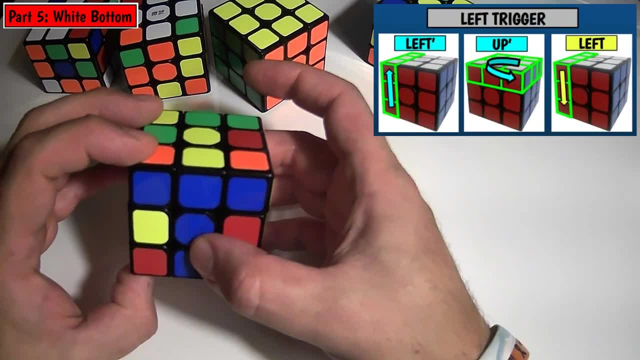 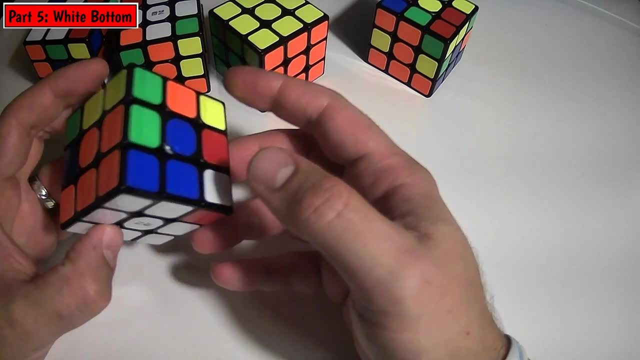 trigger be right there. so to do left trigger. again, we have a left inverted up, inverted left. okay, so there you can see that i'm just down to the one which is right there and again, do not try and twist the pieces now again, i want it to be up. 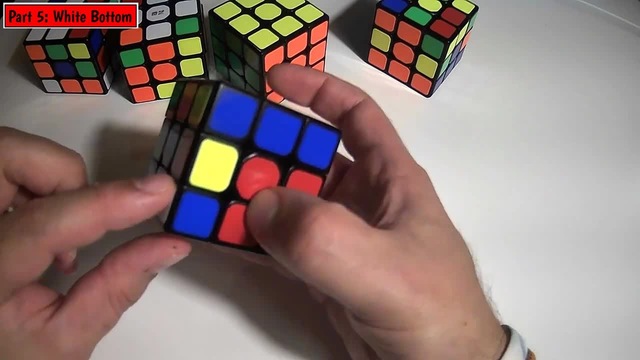 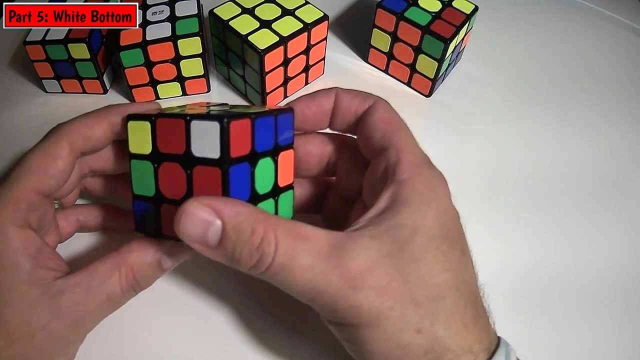 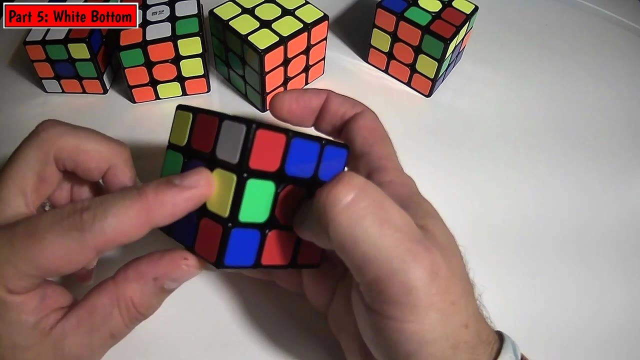 here. so to do that, i'm going to do that left trigger because it's on the left side of my cube. so left, inverted up, inverted left, and now all i have to do is just rotate this top face. so now i've got that diagonal connection: white, red, red because it's on the left side. i'm going. 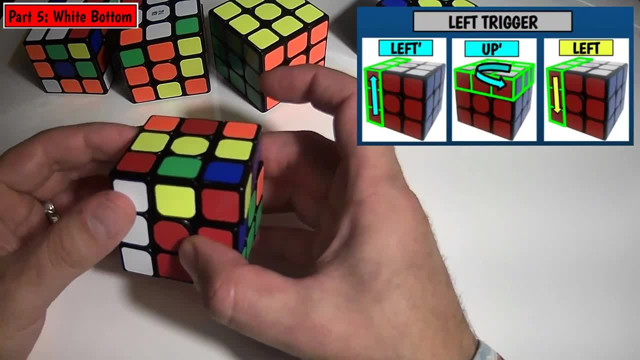 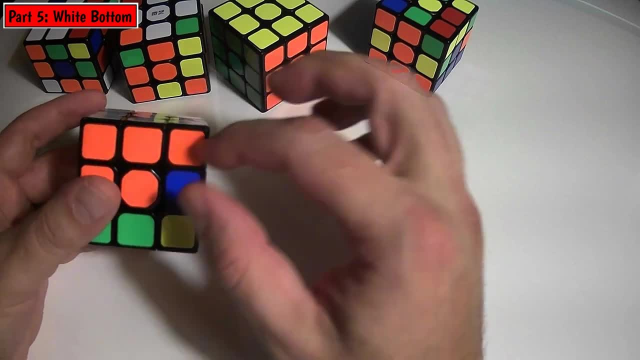 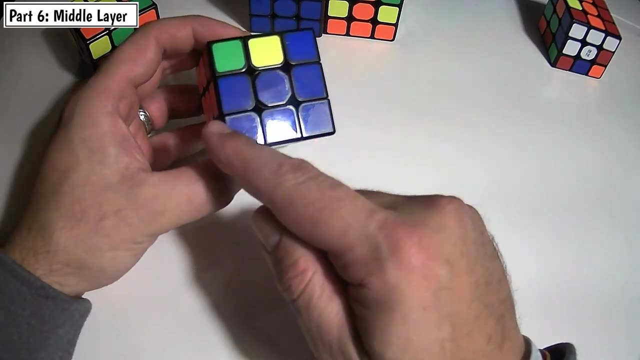 to do the left trigger. so left, inverted up, inverted left, and there you can see that we have made the white bottom and that bottom layer is solved as well. okay, so the next step we are going to try and complete is the middle layer. so you see, the white bottom is done, the bottom layer. 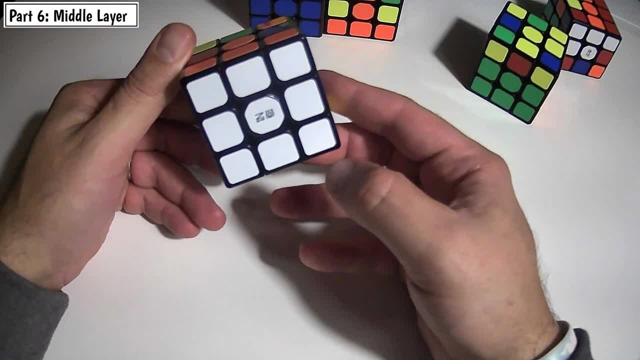 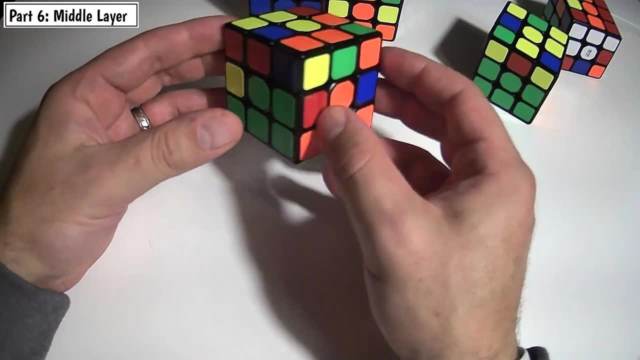 and then the middle layer. so i'm just going to grab this cube that we were working on a minute ago. what I'm going to do is: our goal in this is to place these edge pieces that you see on top where they belong. So, for example, I can see that this is an edge piece that has the border of green. 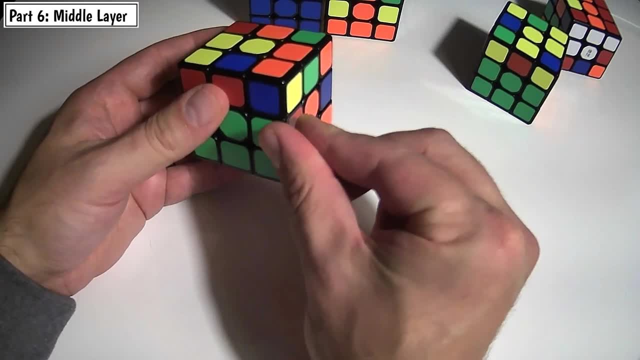 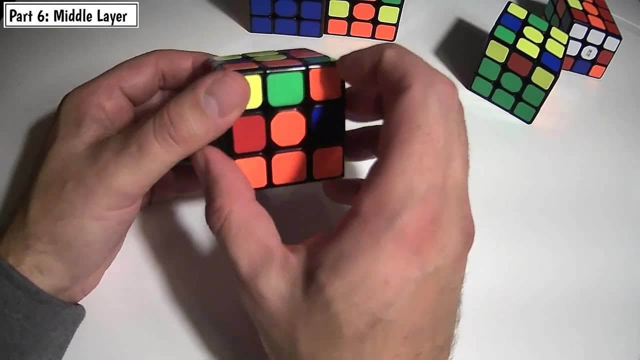 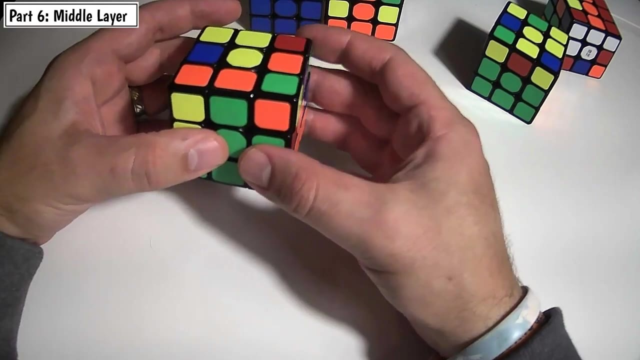 and orange. So I can kind of imagine that that piece really is supposed to go right there, because orange and green are next to each other. So what I'm going to do, I need to rotate this top face until we get this on the right side. So here you can see, the green is all connected. So what? 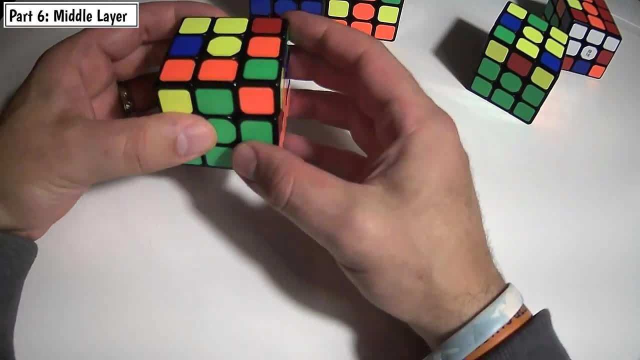 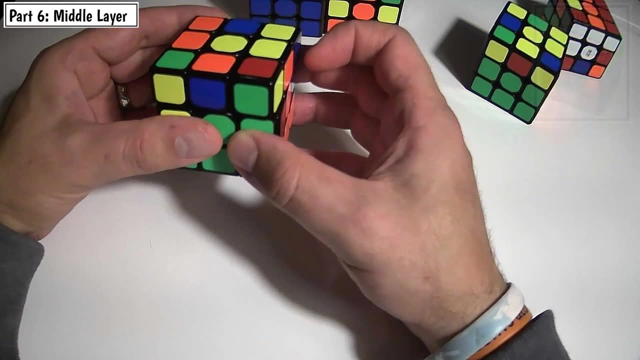 I'm going to do, because this piece, the orange side, is on the right- I'm going to rotate the top face to the right. Okay, so I moved it to the right. Now I'm just going to do the right trigger. 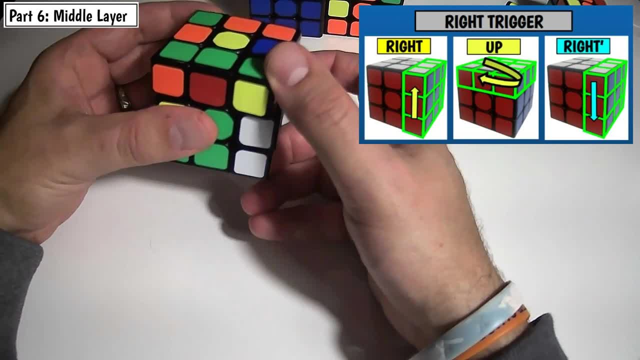 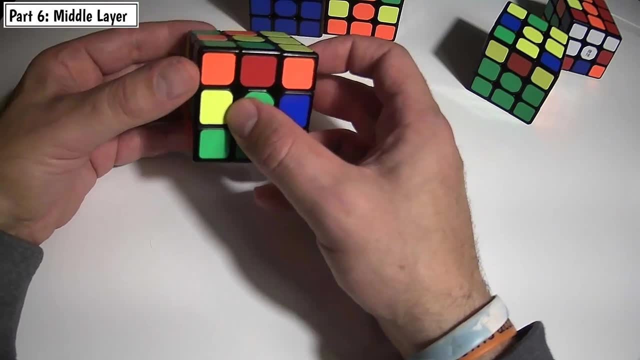 which again is right up, right inverted. Now, because I just moved that white edge piece, I need to get this back to where it belongs. So, just like we did when we were making that white bottom, I need to do the left trigger. 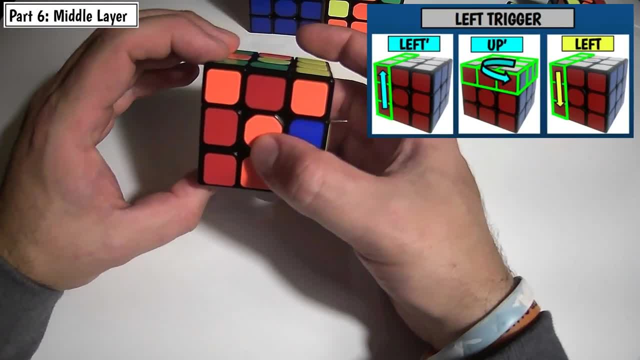 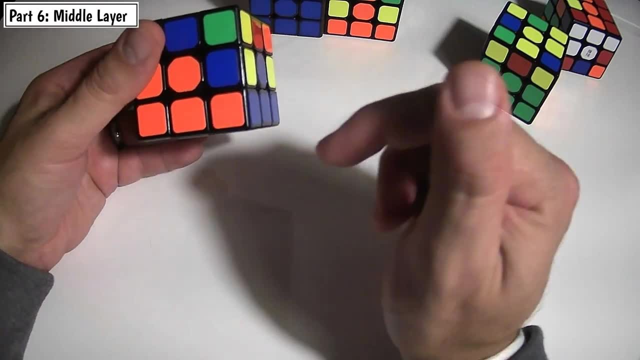 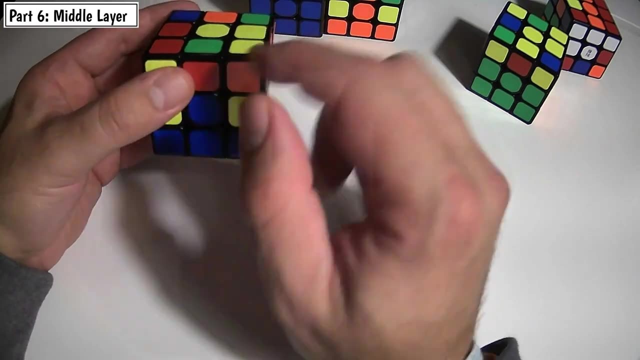 To get this white edge piece back into place. So for the left trigger I'm going to go left, inverted up, inverted left. And now you can see that not only did that edge piece get in the right spot, which was right there, but now we've got the white bottom solved again. 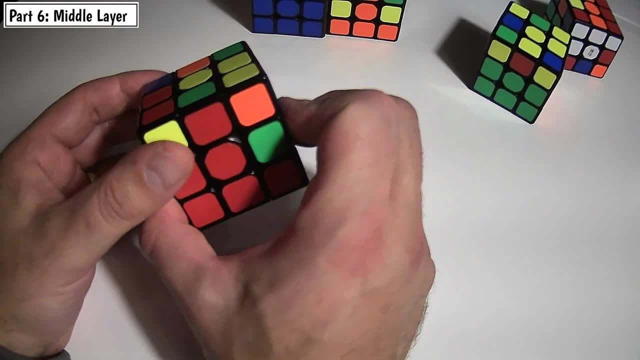 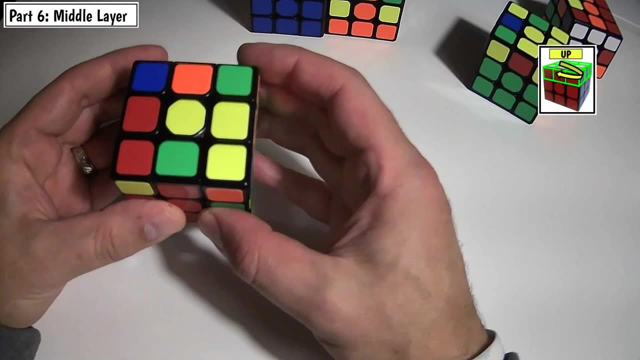 So, to get this guy in the right spot, I'm going to move this to the right. So, now that I've got the reds matched up, and again because the green face is to the right, I'm going to start by moving this to the right. So, now that I've got the reds matched up, and again because this: 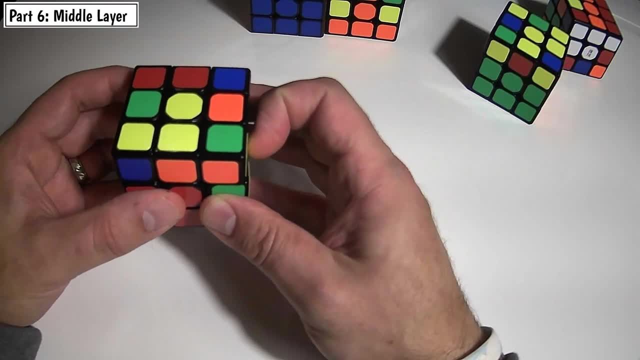 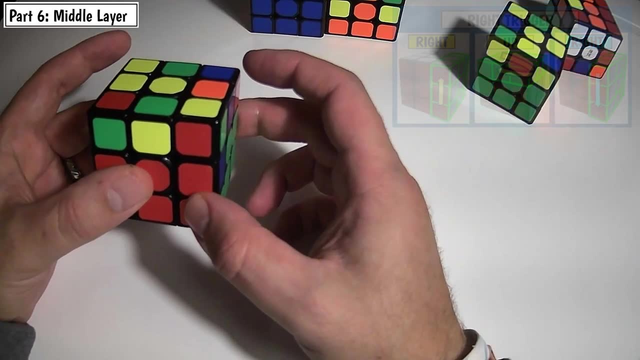 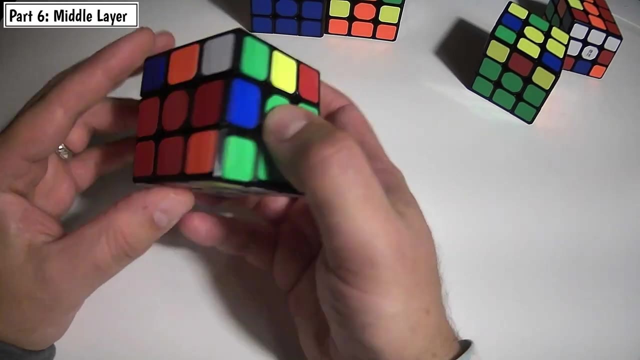 by moving the face to the right, just like this, and then perform that right trigger again. So right up, right, inverted, And I need to put this white sticker back into place, so I'm just going to rotate that diagonally. 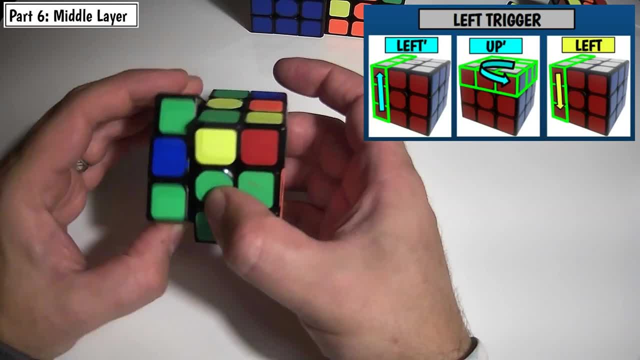 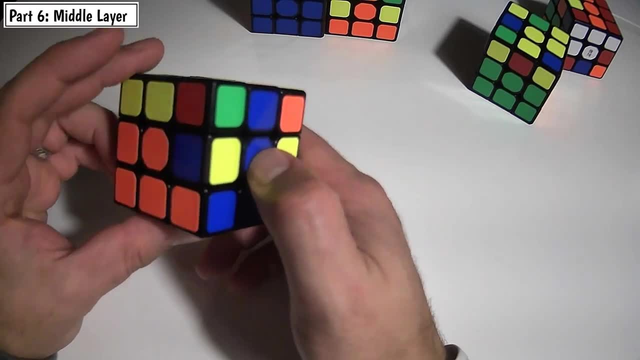 so that it matches diagonally, and then I can do the left trigger. So left, inverted up, inverted left, and there you can see, that's back to normal And we really we're getting closer. We only have a couple more edge pieces. 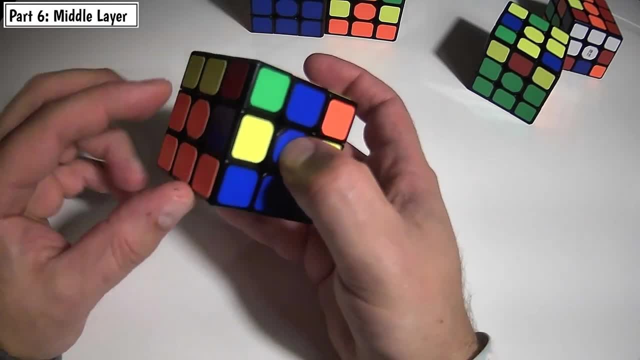 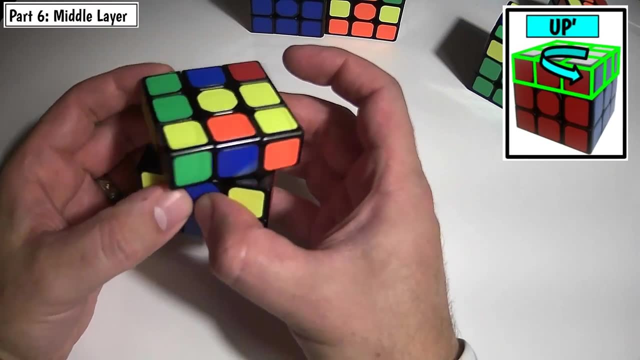 that need to be moved. Okay, so here we've got the orange and blue, which eventually will be right there in that corner. Because this is to the left, I'm going to rotate the top face to the left and then do the left trigger. 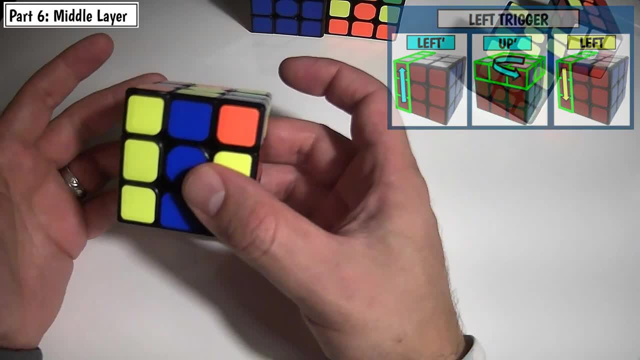 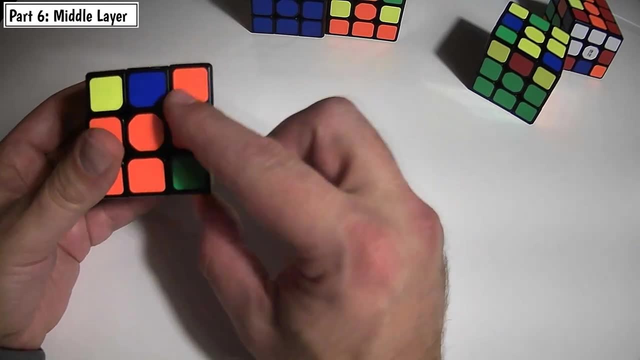 So left, inverted up, inverted left, And again- I know that looks kind of funny right now- I just need to move this orange piece back into place, And so now we've got that matched diagonally and the white is onto the right. 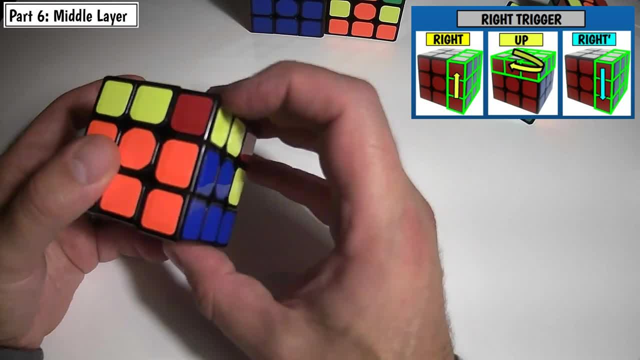 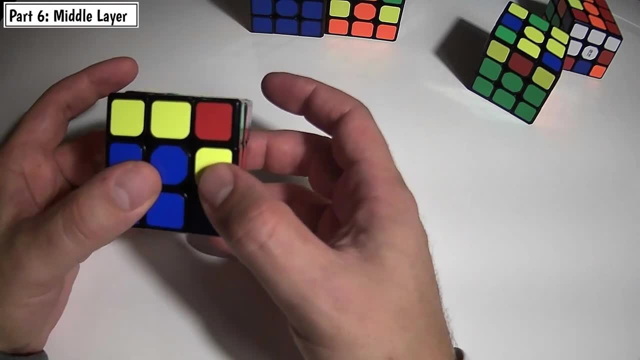 so I'm going to do the right trigger. So right up, right inverted. Okay. so now we're getting closer, So the only piece that we're missing right now is this one, So what I'm going to do. so there is that last red and blue piece. 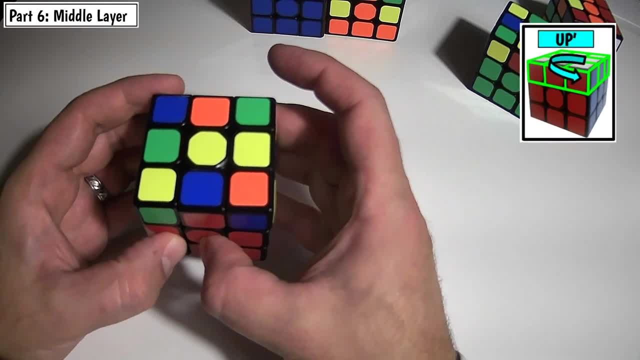 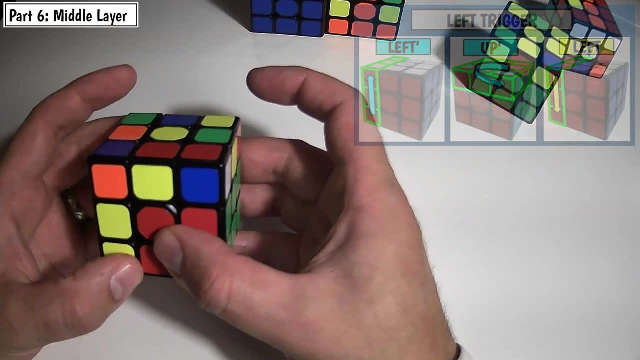 that I need to move here to the left. so I'm going to turn the top face to the left and then do the left trigger. So left, inverted up, inverted left. And don't panic, because we just need to get this white sticker back on the bottom. 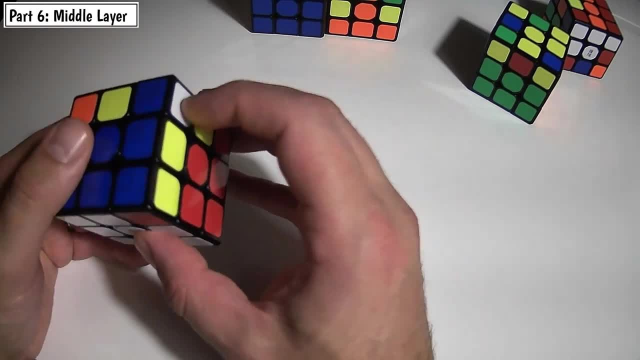 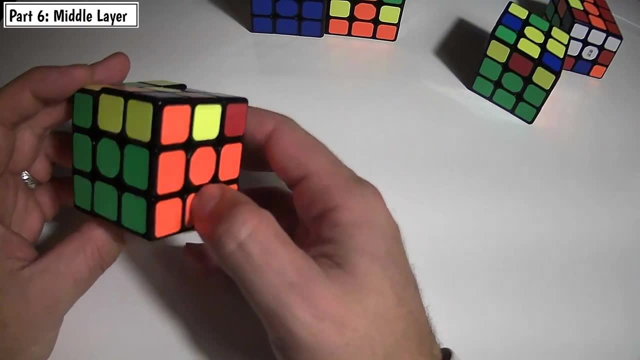 There we see that diagonal connection again. So white's on the right. so I'm going to do the right trigger which is right up, right inverted, And there you can see that we have made the middle layer All right. now I want to explain one more little issue. 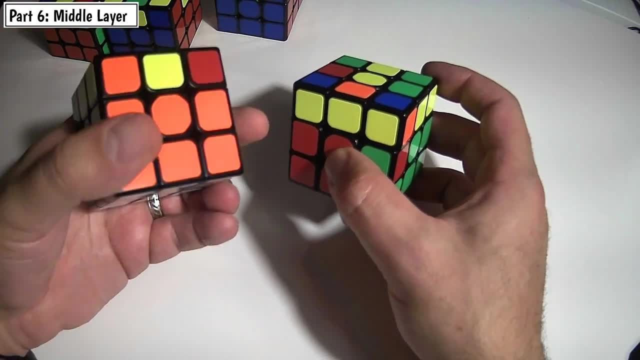 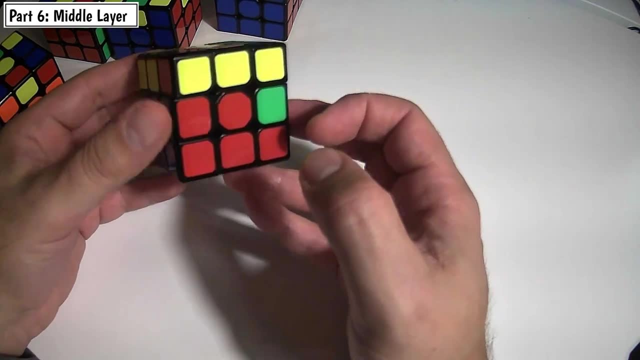 that sometimes comes up with the middle layer, that I did not encounter when I was just modeling it on this one. So you can see on this cube right here you can see that I'm almost done with the middle layer, except for this piece right here. 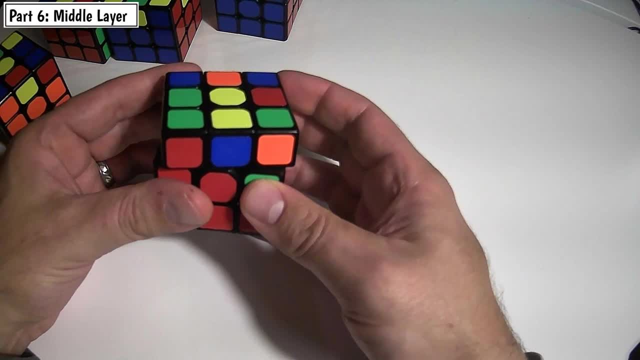 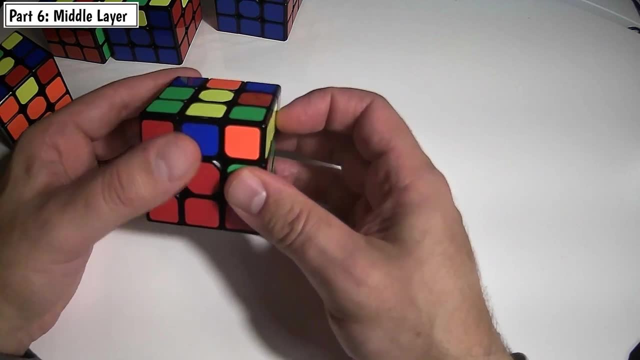 And if I look through all of the pieces on top, you can see that all of the pieces that are remaining have yellow right. You see how there's yellow, yellow. So I do not have the piece that I'm looking for on top. 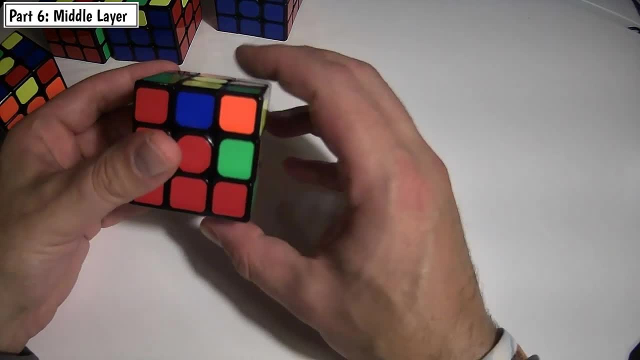 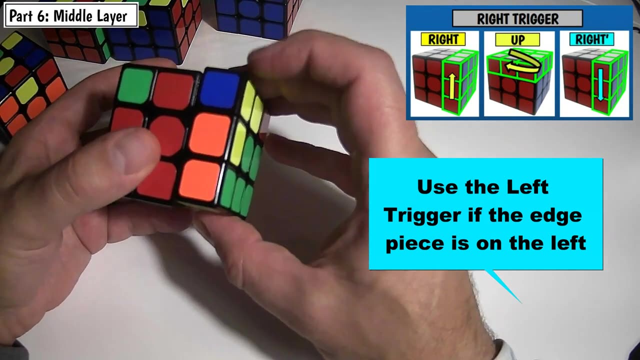 that is going to be that green and red. So to fix this issue- you guessed it- all we have to do is the right trigger. So if I do, the right trigger again, so right up, right inverted, and then the white corner piece back in place. 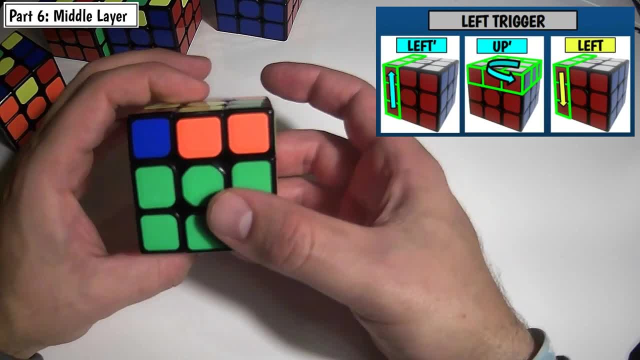 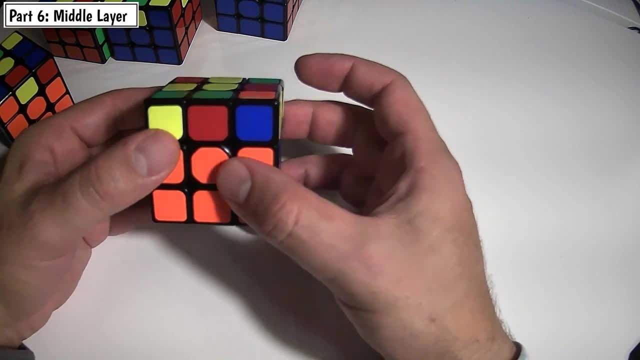 So I got that lined up diagonally. This time around I'm going to do the left trigger, Okay, and now, because I did those sequence of events, now you can see that I actually do have a edge piece here that does not contain yellow. 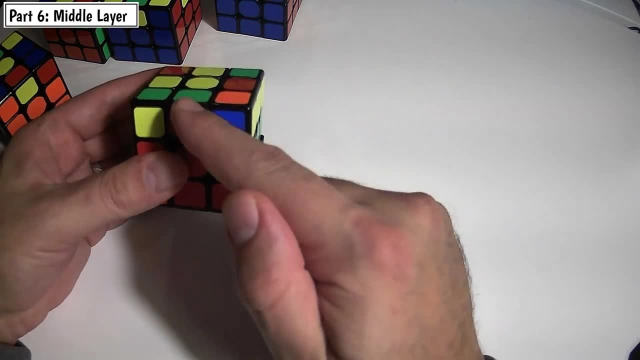 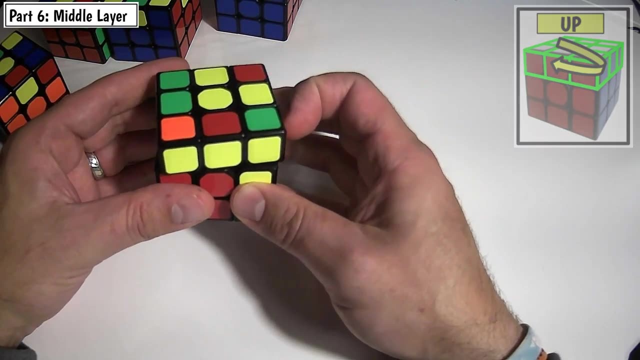 So now I can rotate this And again. so this edge piece needs to go right there. So, because I'm moving that to the right, I'm going to turn this face to the right and then I'm going to do that right trigger again. 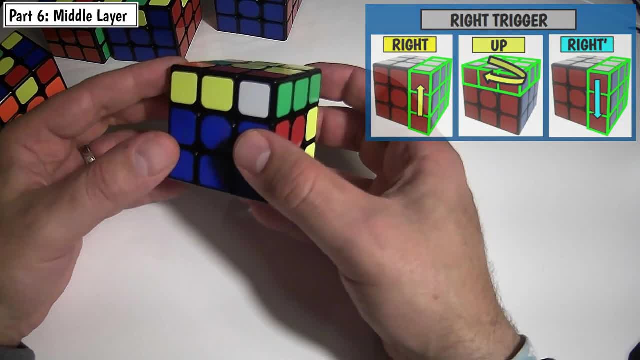 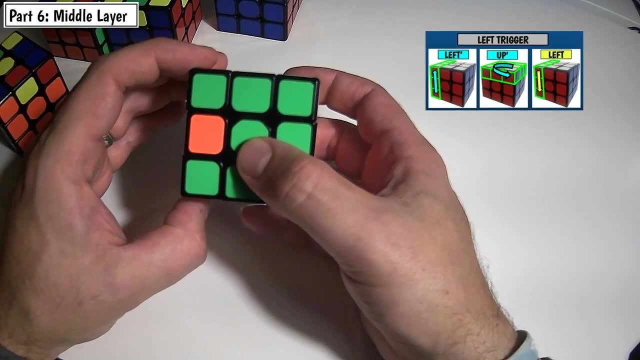 So right up, right inverted. Of course you need to put this white corner piece back into place. So I go like that: match those up diagonally and then I can do the left trigger again. So left inverted up left. 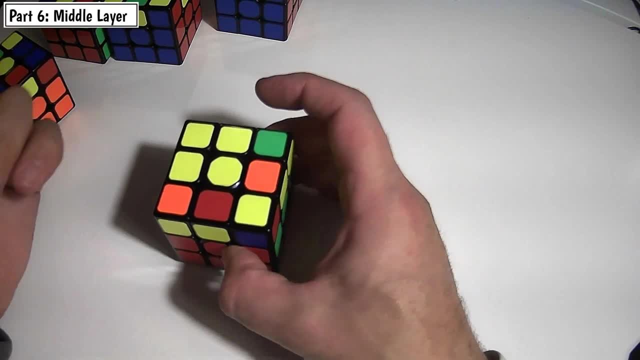 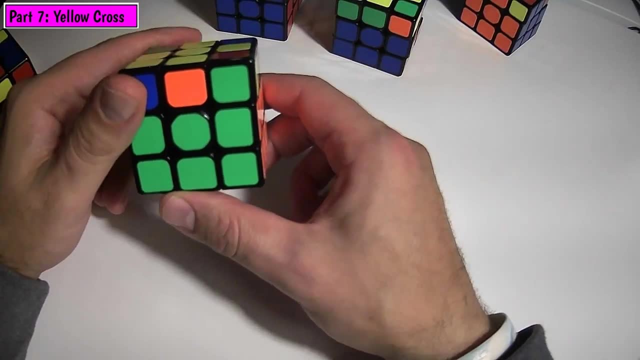 And again, sometimes that happens- You'll see different variations when you're solving a cube. Sometimes you might have to do the algorithm more than once, but that is an issue that sometimes we encounter with the middle layer. All right, so the next step that we are going to practice. 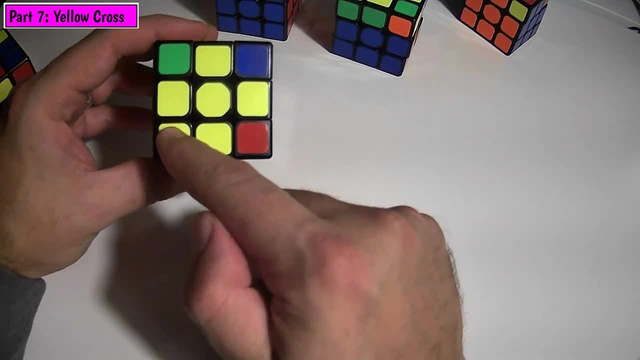 is making the yellow cross, So you can see yellow cross and in this case I actually had an extra one in place. So I'm going to do that. I'm going to do that in place, but we're going to try and make the yellow cross. 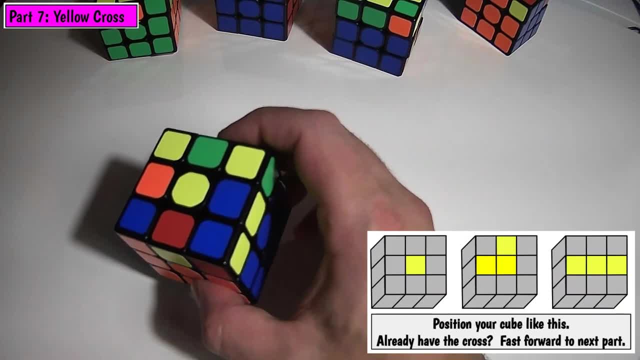 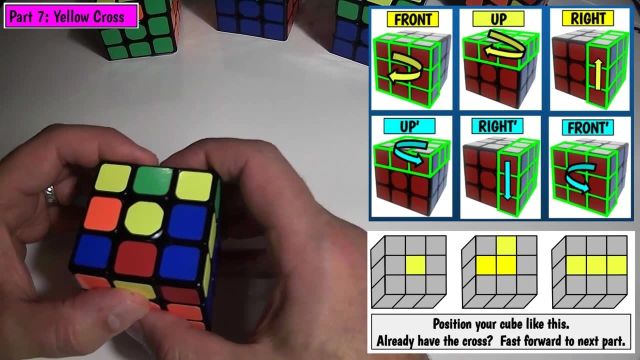 So to perform this- this is really the first algorithm we're going to see today. that is not the right or left trigger, And so you can see the algorithm up here on the top. Some people like to call it fur-erf, As you see these letters. 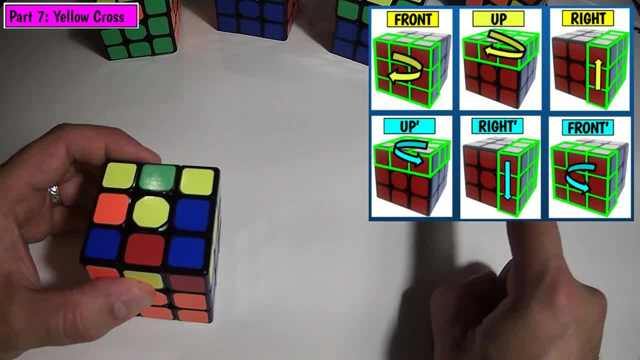 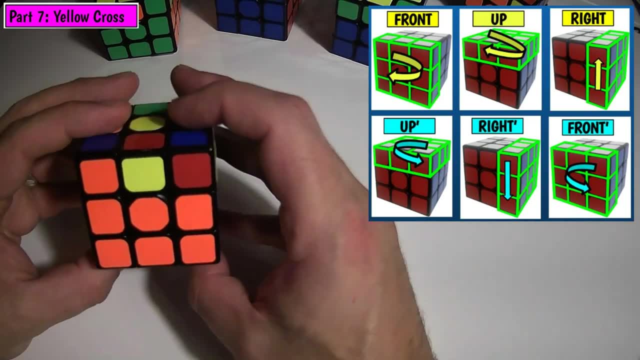 you know, it kind of spells out fur-erf, And the first three moves are just the regular moves And then the blue moves, where you see the blue arrows, are the inverted moves. So let me model that. So I'm just going to hold it just like this. 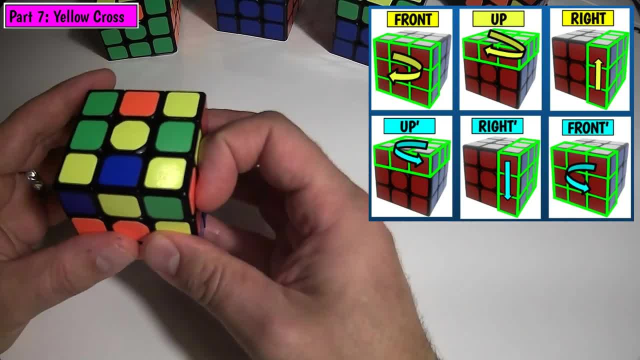 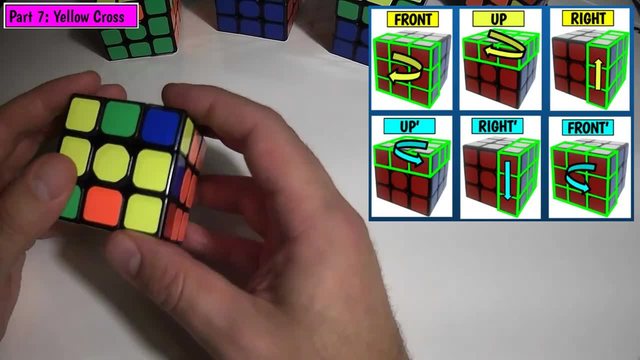 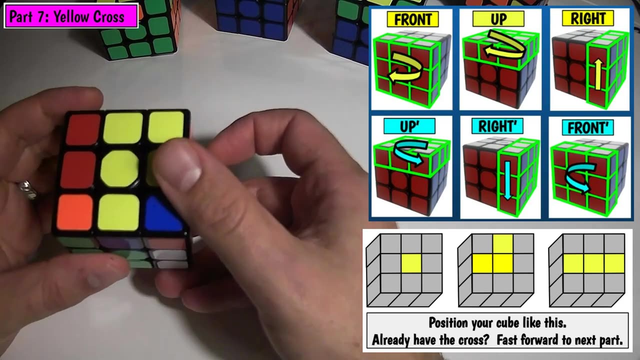 So I'm going to go so: front up, right up inverted, right inverted, front inverted. Okay, so that did not work the first time, Let me do it again. So we have front up, right up, inverted. 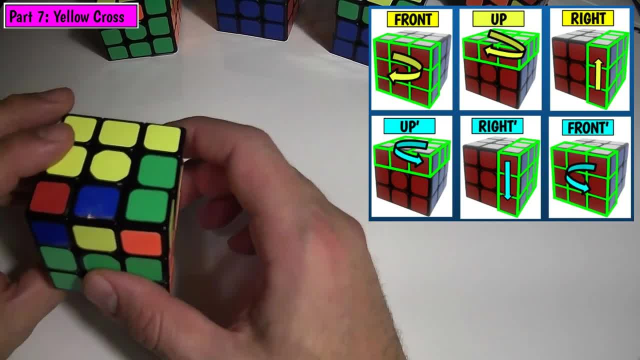 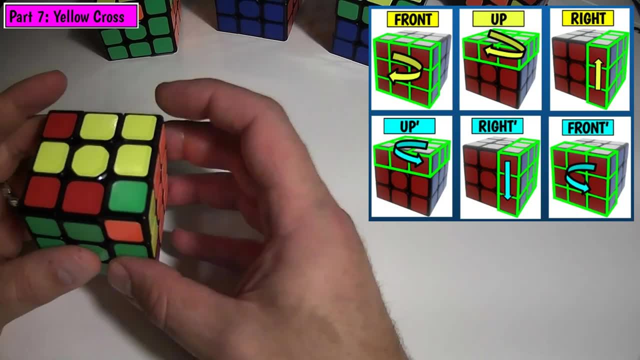 right inverted, front inverted. And there again, sometimes you're going to have to do these algorithms more than once. So front up, right up inverted, right inverted, front inverted, And there we can see that we've made the yellow cross. 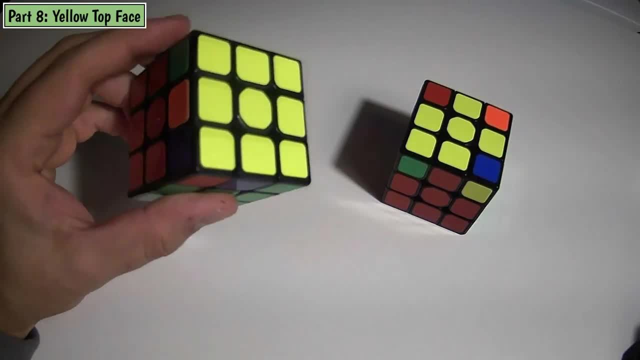 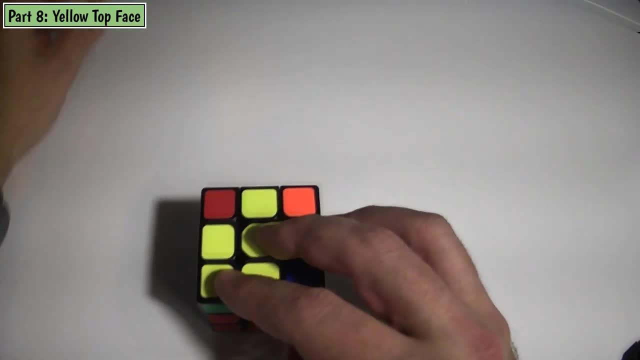 All right. so the next step we are going to try and do is making the entire top yellow face. Now, depending on how your cube looks, you can see I've got some pictures up here on top Match. try and find how you have the yellow cross. 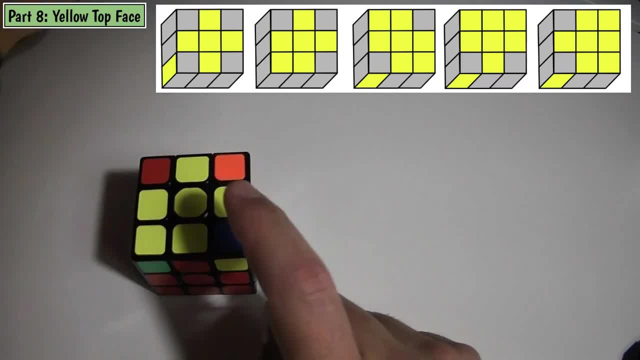 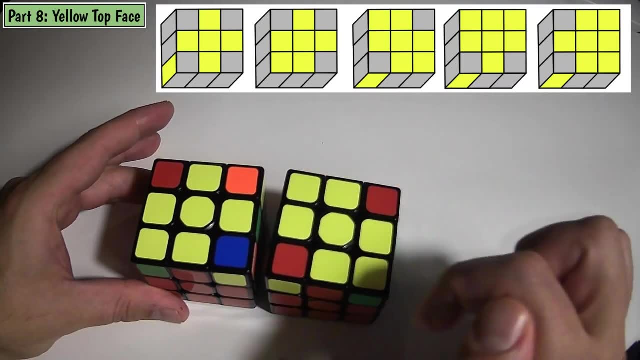 made on yours, because sometimes you might have a cube that looks like this. You might have a cube that looks like this, where you still see the yellow crosses, but you can see there are also some, you know, yellow corner pieces that are also in different spots. 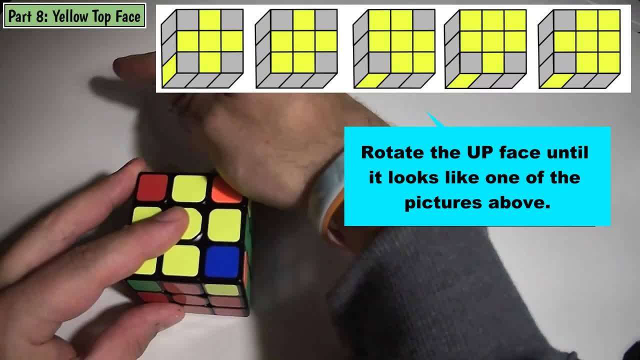 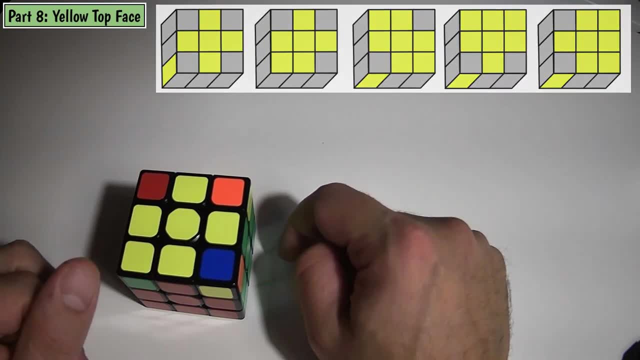 So again, before you proceed into actually doing this algorithm, try and find which picture it matches and positions a cube, just like you see in the picture. Okay, so now we've got another algorithm that we are going to learn, but to perform this algorithm? 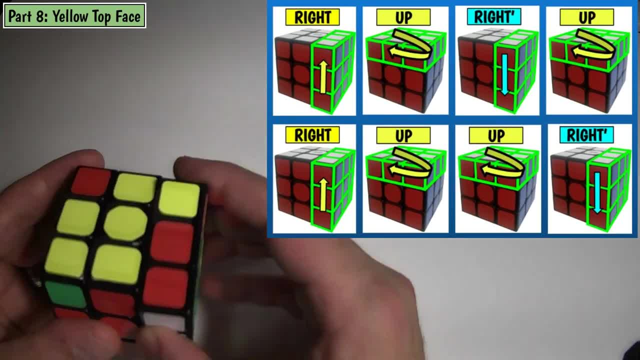 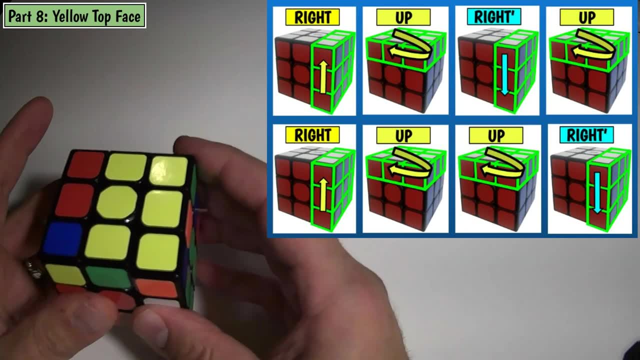 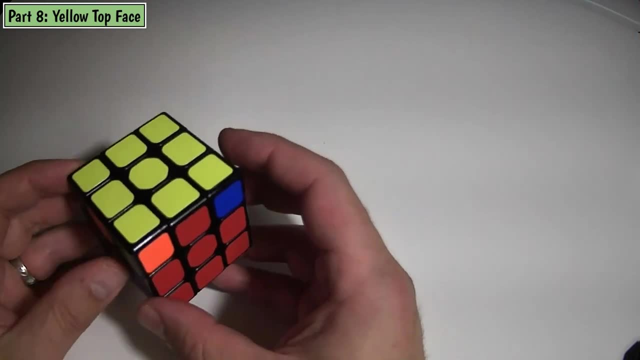 what you're going to do is we're going to do start with the right trigger, So we have right up, right inverted up, right up up, right inverted, Okay. so in that case I got really lucky. 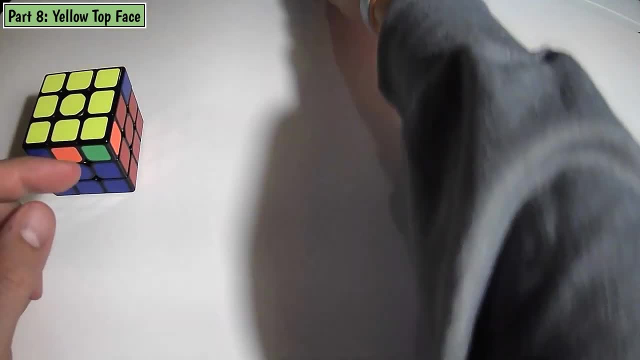 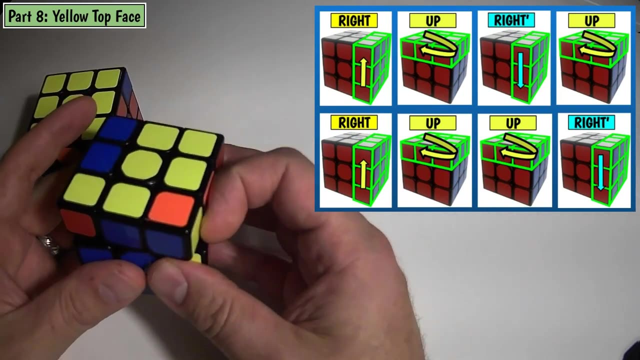 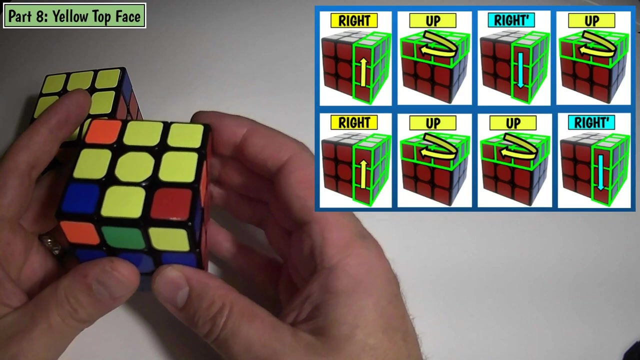 I only had to go through with that algorithm once. Let me try it with another cube to see if I get lucky again. So we have right up, right, inverted up. right up up, right, inverted. Okay, so that did not work. 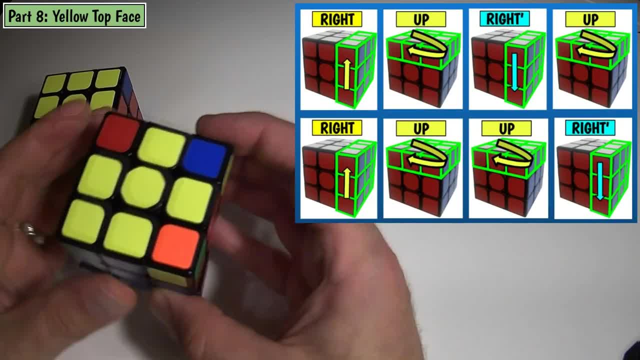 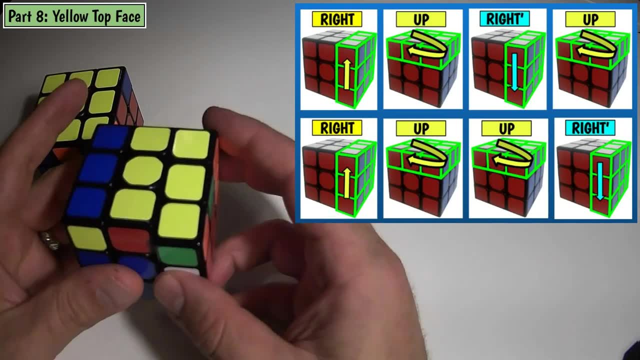 So I'm going to do this again and I'm going to position this So it kind of looks like the fish is down there in the corner. So we have right up, right inverted up, right inverted, Right inverted up, right up up, right inverted. 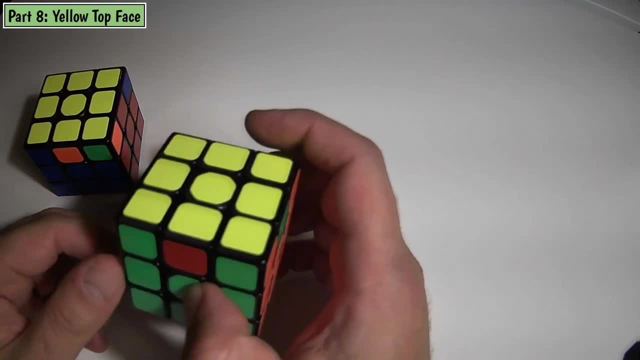 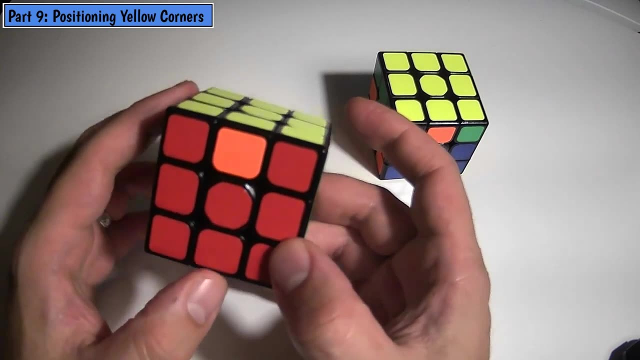 Okay, so that actually did work out. So again, it's going to depend. Sometimes you might only have to do the algorithm once, Sometimes you have to do it twice or maybe even three times. All right, so the next step we were trying to do: 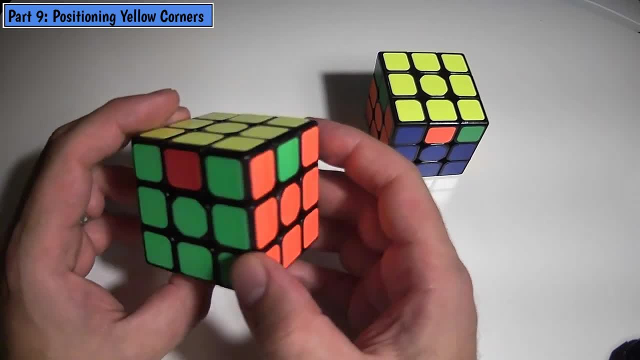 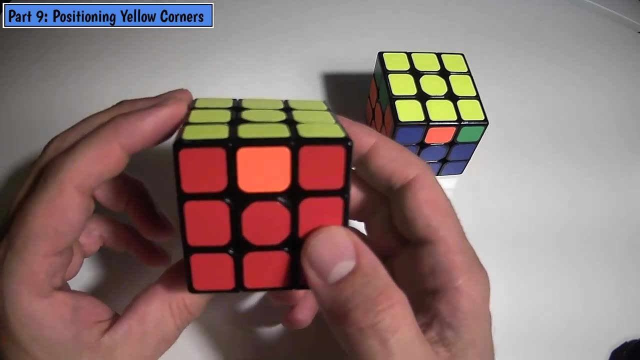 is. we were trying to position the yellow corners correctly. Now I just modeled doing the yellow top face, and this I could actually skip over With this cube right here. there's an entire step we don't have to do, But our goal. 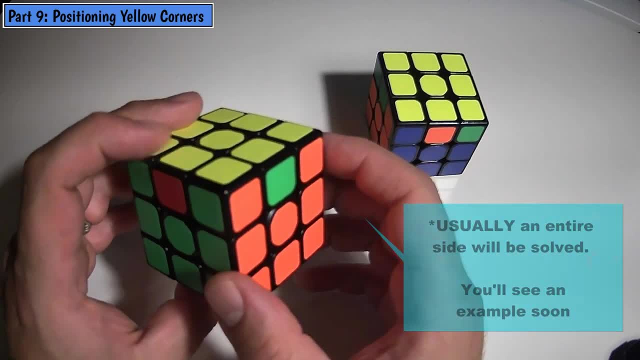 after we do this step is we're going to have one. the one side's going to be completely solved, and then we're going to get these yellow edge pieces in the right spot. Okay, so the next thing that we are going to do, 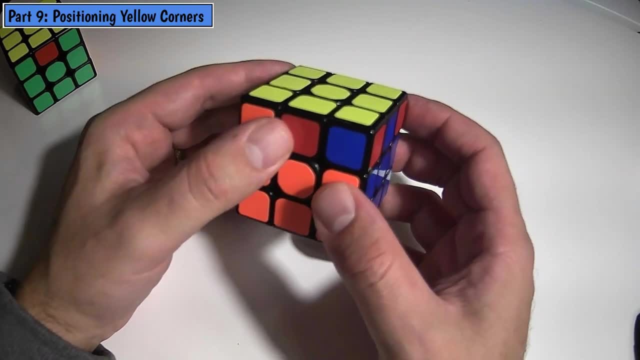 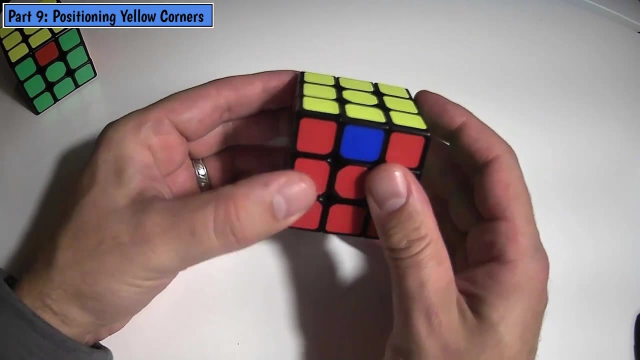 is we're going to position those yellow corners to make sure they're in the right spot. So what I'm going to do is I'm going to kind of rotate the top face around until I get some corner pieces that match. For example, we can see there: 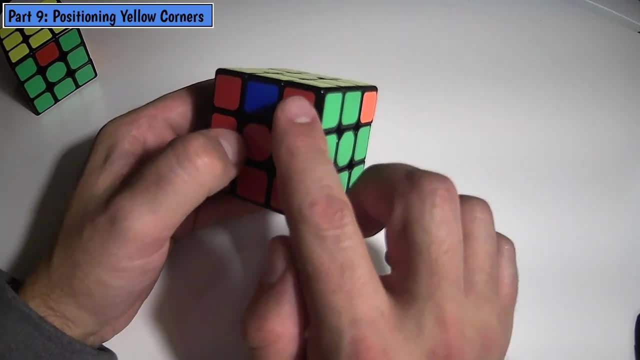 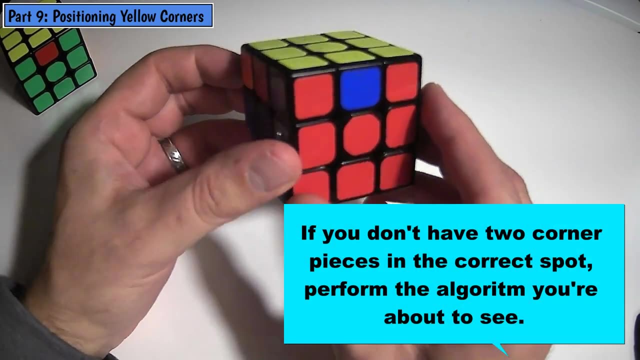 that I know that these two red corners are in the right spot, because red matches green, We can see that blue matches red, So I've got those in the correct spot. So what I'm going to do is I'm going to turn this so that that is away from me. 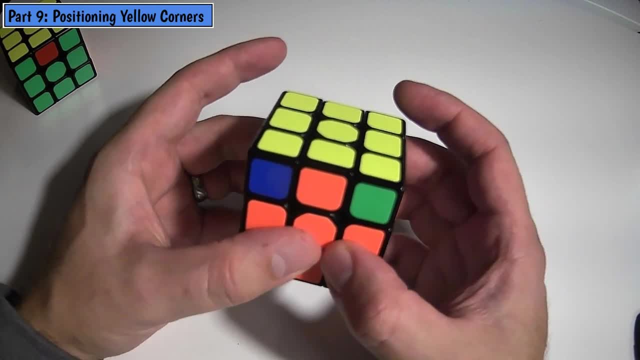 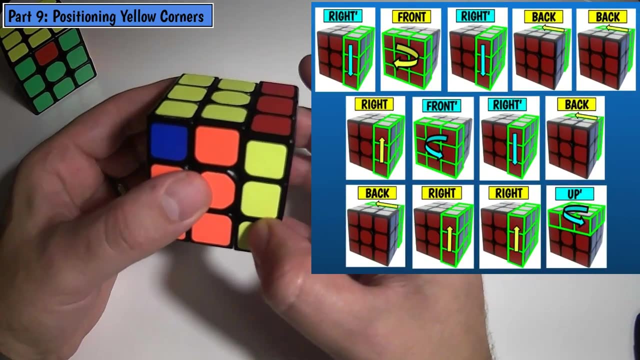 You can see that that is away from me. And then I've got a soup- probably the longest algorithm we're going to see today to position these yellow corners correctly. So I'm going to start by doing right inverted front: right inverted. 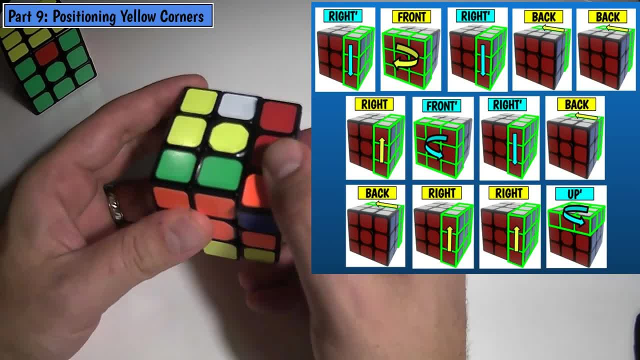 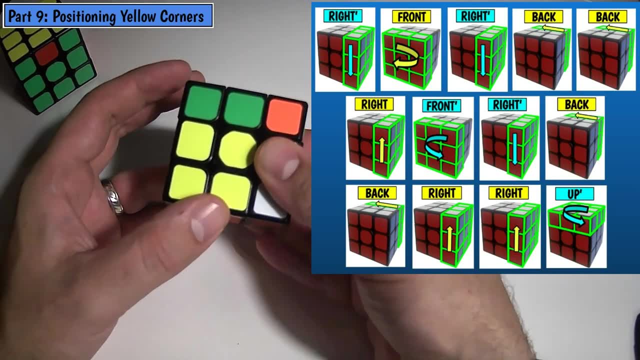 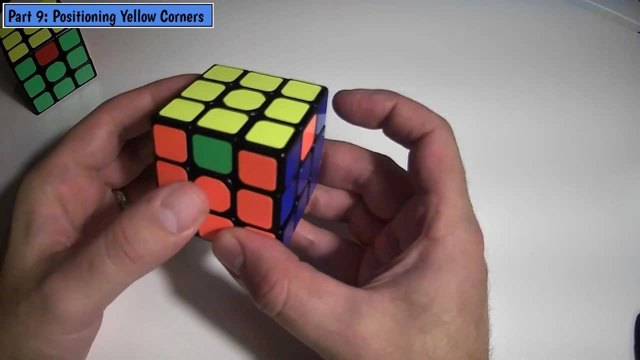 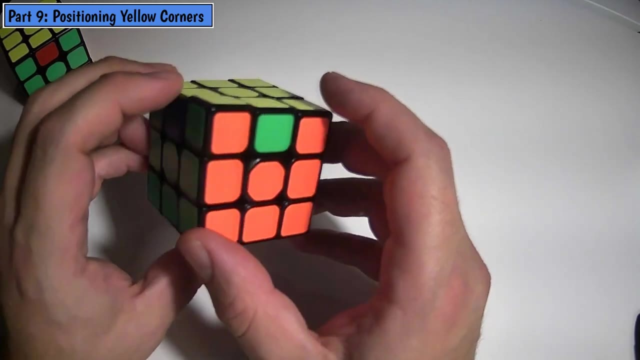 back back right front, inverted right, inverted back back right, right up. So now you can see that we've got one side completely solved and we've got all of those yellow corners now in the right spot. Okay, so before I show you the next algorithm, 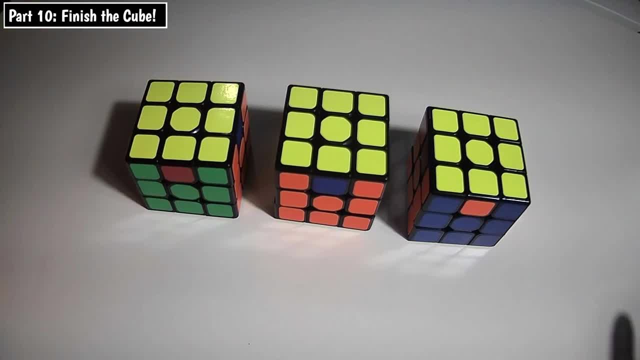 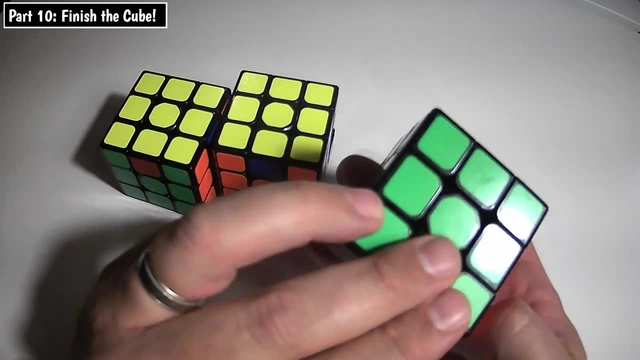 to complete the entire Rubik's cube. you've got to take a look at your cube and figure out which puzzle you need, because on each of these three they're slightly different. So from this one, for example, we can see the green face is already done. 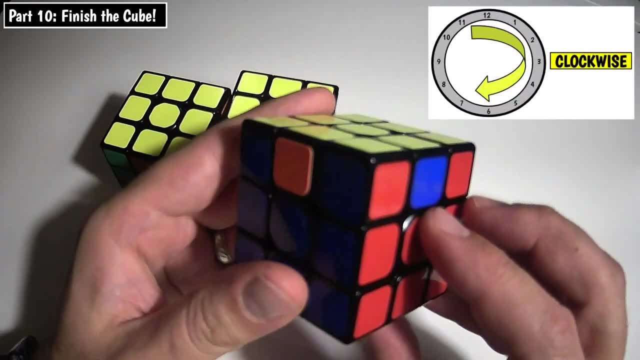 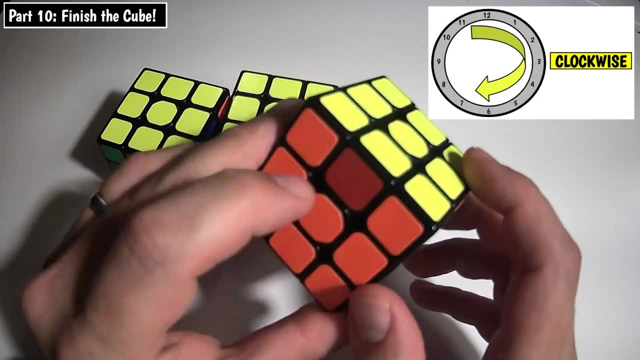 and we see that there are three edge pieces that need to be moved. In this case, this blue and yellow edge piece really needs to go right there, And this orange and yellow piece really needs to go right here. On this one, it's the opposite. 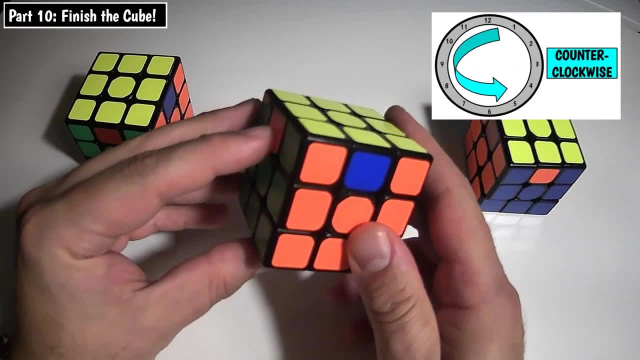 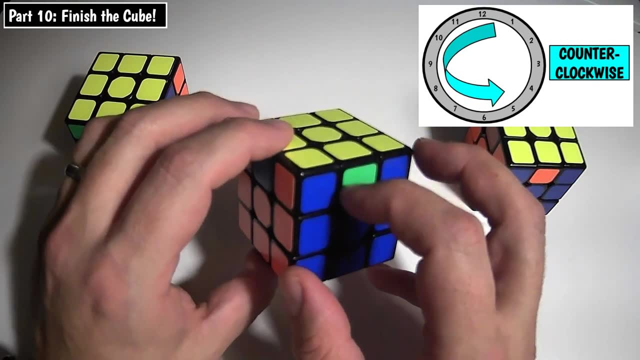 where I've got the red side. that's completely done. but this time around, this orange and yellow piece needs to move to the, and then this blue and yellow piece also needs to move to the right, And in this last cube you can see that all of the yellow corner pieces are in the right spot. 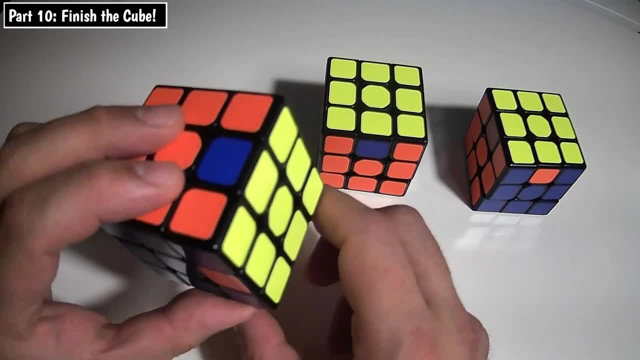 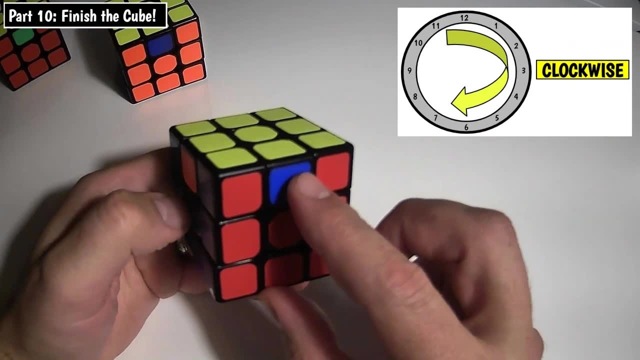 but I don't have any sides that are completely solved. So in a situation like this, you can actually pick either of the algorithms to try, All right. so I'm going to start with this cube, because these pieces need to move to the left, this one needs to move to the left. 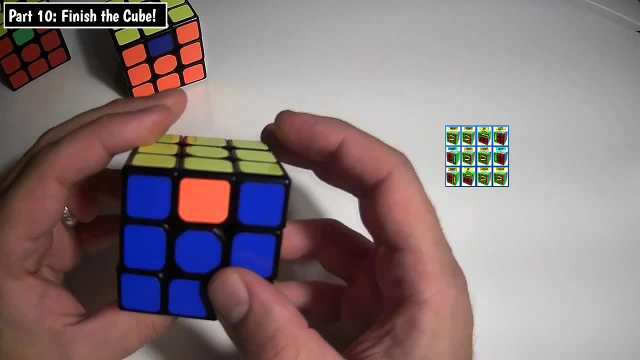 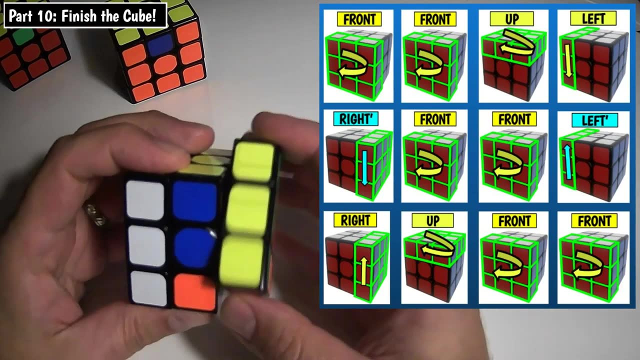 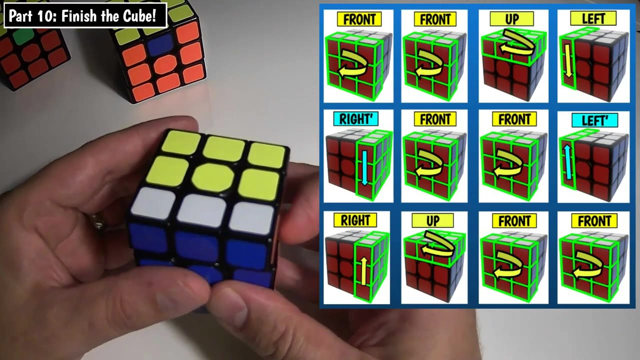 So if you need to move those edge pieces to the left, you can follow this algorithm. So we have front front up left, right inverted front front, left inverted right up front front, And there you can see that this cube is completely solved. 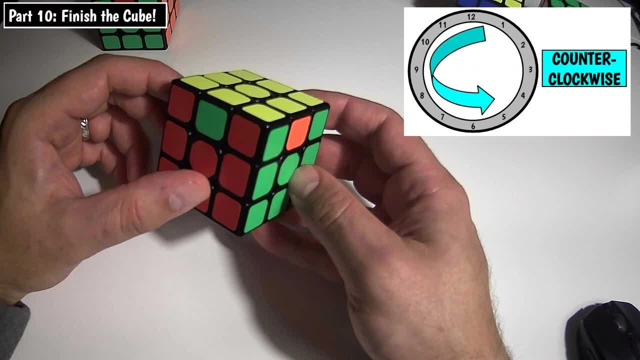 Okay, so you can see on this cube it's slightly different. You're going to see, the algorithm is nearly the same. there's just two little small differences. So this time around I need to take this yellow and green edge piece and move it to the left. 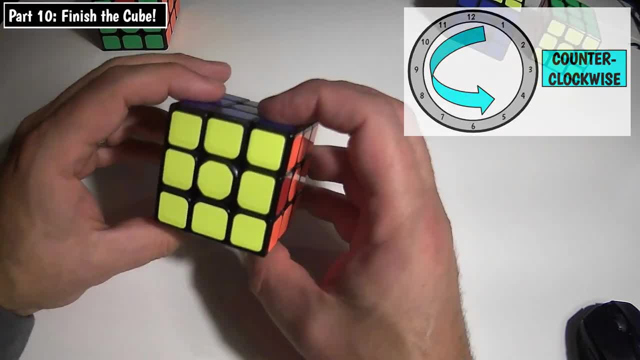 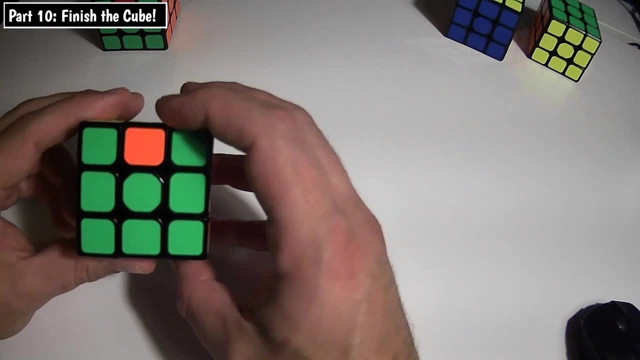 And this orange and yellow piece needs to move to the right. This back blue face is completely done. So you're going to see just a slight difference in the algorithm. we just did So to get those edge pieces to the right. we're going to follow this algorithm. 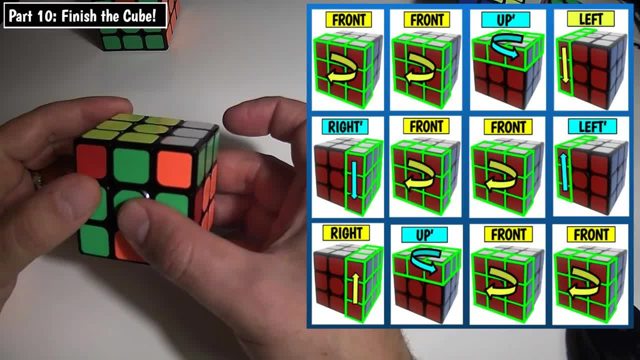 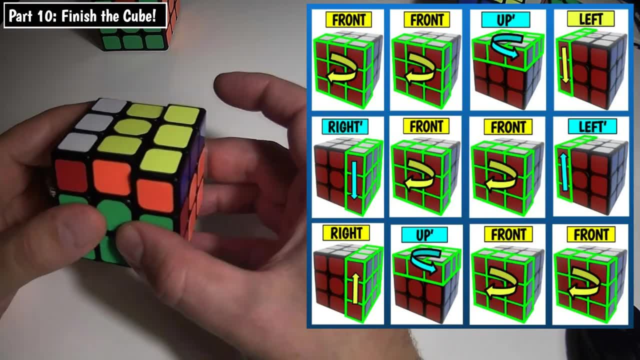 So we have front front up inverted, left, right inverted front front, left inverted right, up inverted front front, And there you can see that this cube is also moving to the right And this cube is also solved. 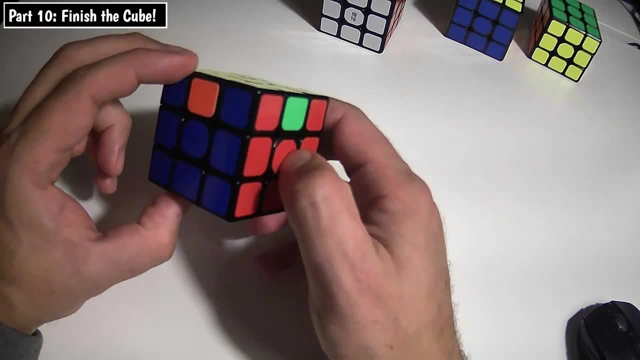 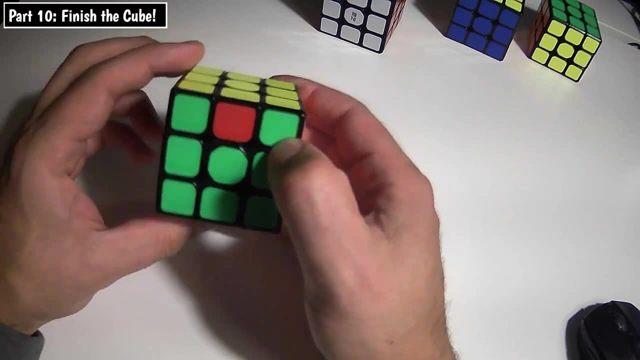 Now, in this example- this was the weird one that I was showing you a minute ago- where, in this one, none of the sides are completely solved. In this case, you can see that this needs to move to the right and this needs to move to the left. 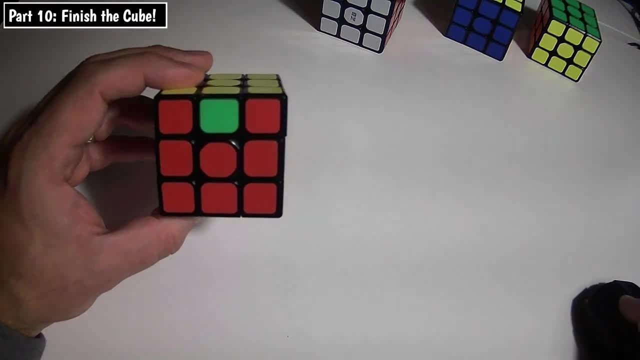 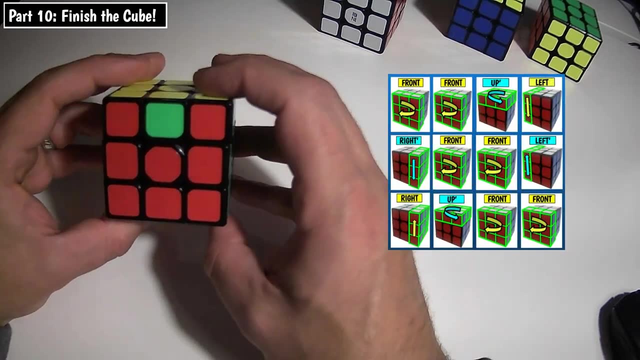 So, to be honest, you can really pick either of the algorithms, because you've got some that need to go to the left and some that need to go to the right. So I'm going to start by just performing the algorithm you see on the screen. 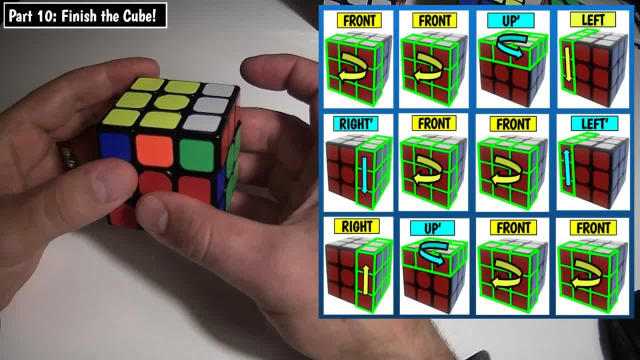 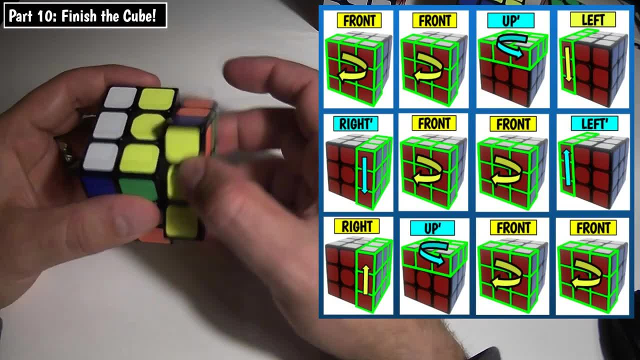 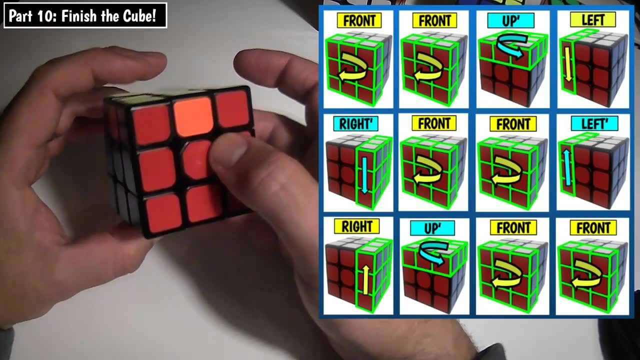 So we see front front up and left Up inverted left, right inverted front front. left inverted right up inverted front front. So now you can see that we've got one side completely solved And then for the pieces that are remaining, you can see this one needs to move to the left.